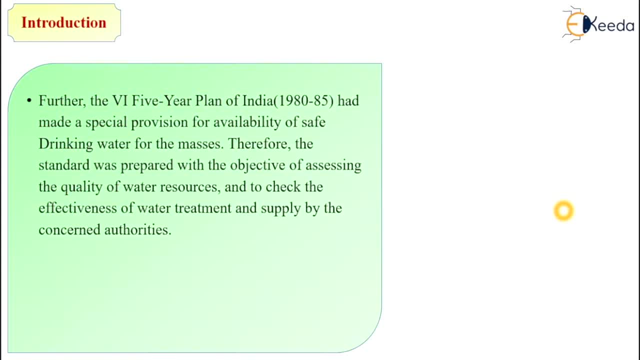 The measurement was very important for the quality of water and to check the effectiveness of water treatment and supply by the concert authorities. Routine surveillance of drinking water supplies must be carried out by the relevant authorities to understand the risk of specific pathogens and to define proper control procedure. 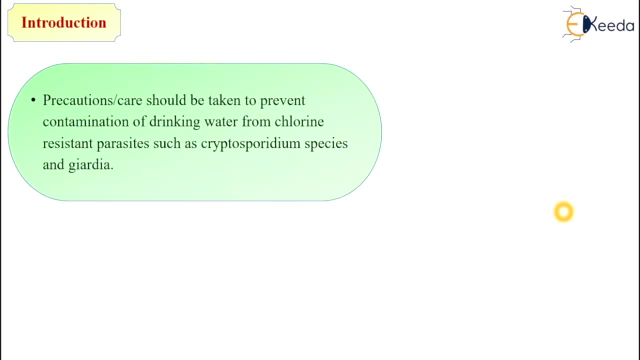 Precautions or care should be taken to prevent contamination of drinking water from chlorine resident parasites such as Cryptopyridium species and Gyredulia. So these are some bacteria species which make water make unsafe for drinking. So what is safe? water which is free from pathogenic agent and harmful chemical substances. and 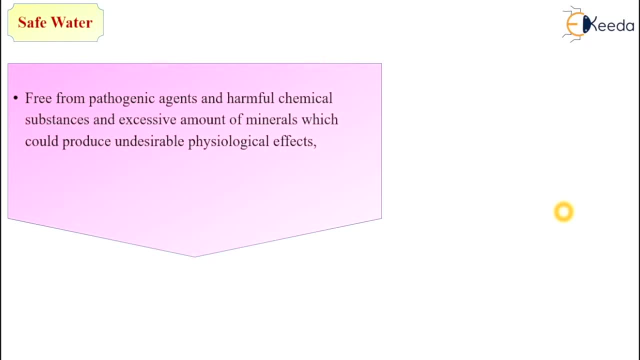 excessive amount of minerals which could produce undesirable psychological effect. So that water we called it as safe water and which is pleasant to the taste, that is free from color and odor and also usable for domestic purpose, So the water which fulfills is safe water. 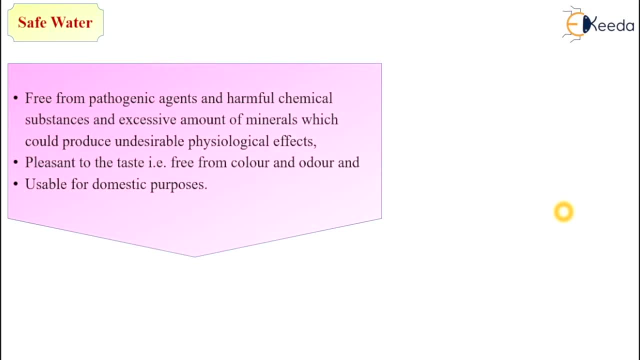 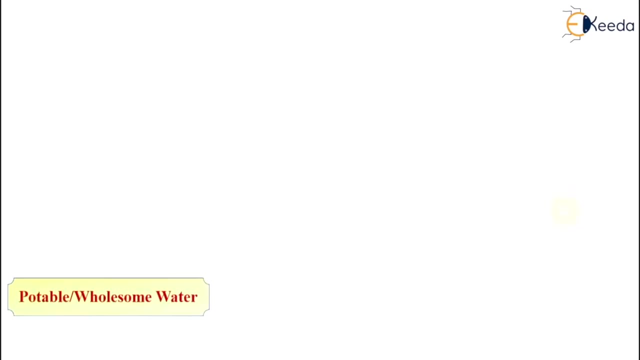 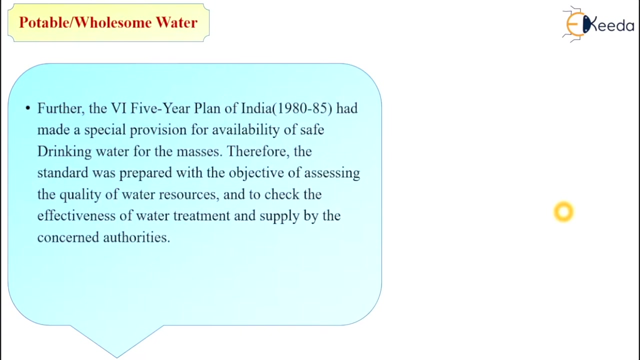 So what is required? criteria, that is, that are: it is free from pathogenic bacteria, it is free from odor and color and it is also useful or usable for domestic purpose, So that water we can called it as safe water. So what is potable or wholesome water? further, the 6th 5 year plan of India had made a special provision for availability of safe water. So what is potable or wholesome water? further, the 6th 5 year plan of India had made a special provision for availability of safe drinking water for message. So what is potable or wholesome water? further, the 6th 5 year plan of India had made a special 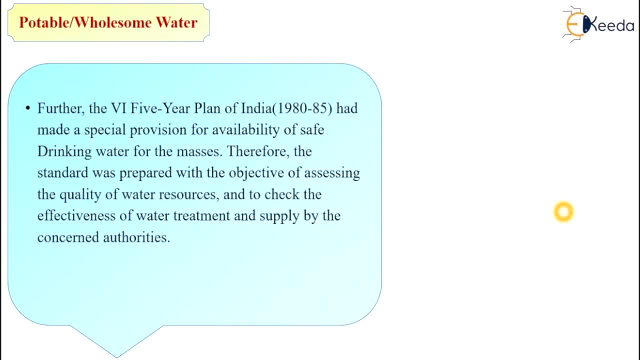 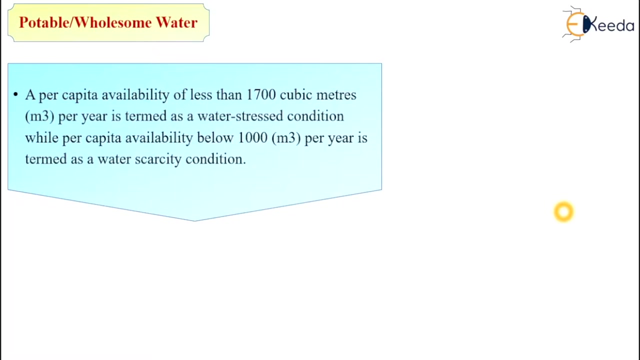 provision for availability of safe drinking water for message. Therefore, the standards were prepared with the objective of assessing the quality of water resources and to check the effectiveness of water treatment and supply by the consent authorities. So safe water, pleasant to taste, odor, colorless and does not stain cloths and utensils. 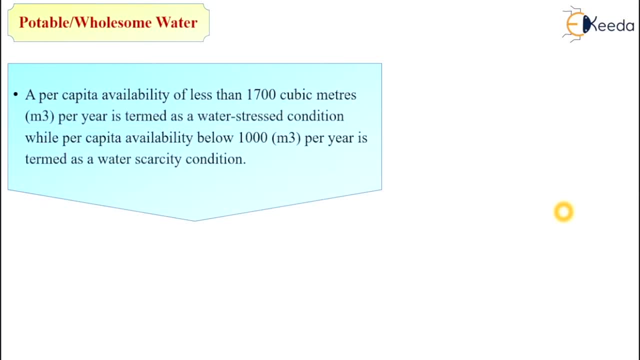 But what is potable or wholesome water? further, the 6th 5 year plan of India had made a special provision for availability of safe drinking water for message, And now they say probably there are 7 topic. one thing: what is the broadly�둘 sing about? 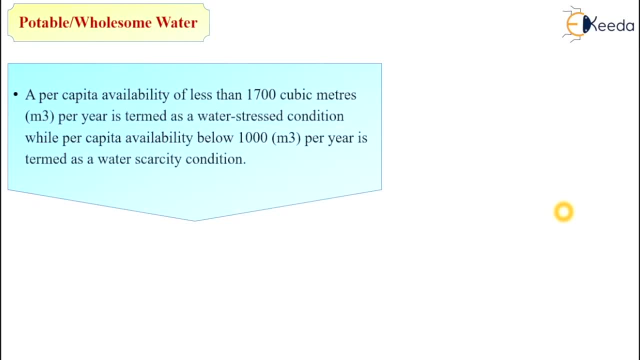 safe drinking of drinking water from a plastic bottle of ice cream dispenser. So much of amateur will go into it. but especially the first one is: won't come out And let's see what is thereו. what's for it? There will be screw to it, and for potable and wholesome water it should don't include. 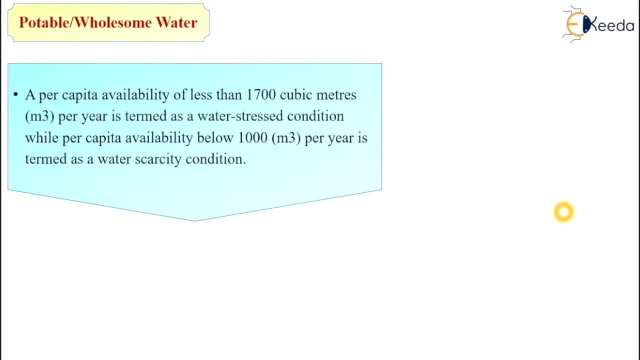 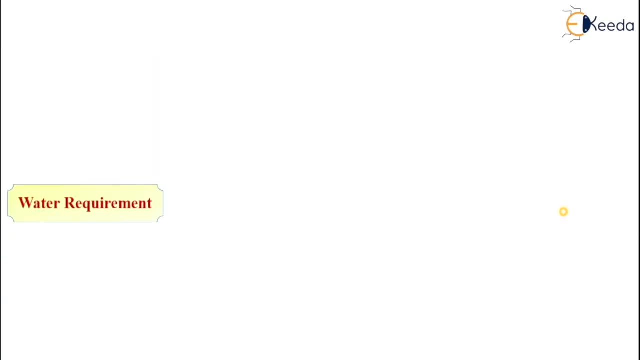 on it. so I've have used to avoid that so that what I had said before, you can want it below the 1000 m3 per capita per year, then we can call it as there is a problem of people facing problem of water scarcity. 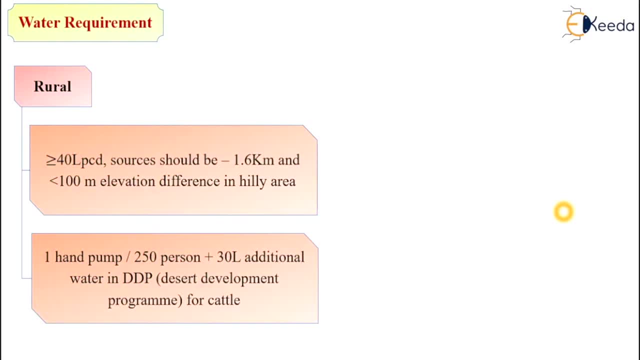 So water requirement: in rural area greater than 40 L per capita per day water is required. sources should be 1.6 km apart from the residential area and less than 100 m elevation difference in hilly area. So for that one hand pump is required for every 250% plus 30 L additional water in desert. 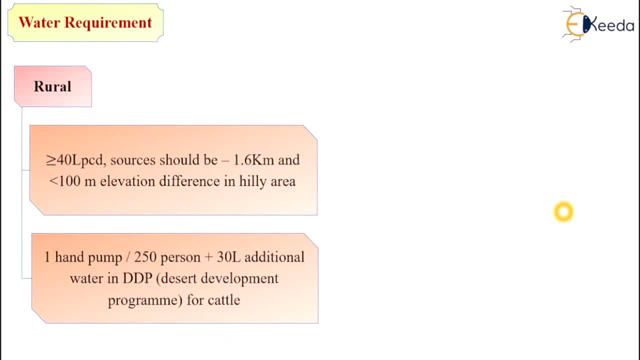 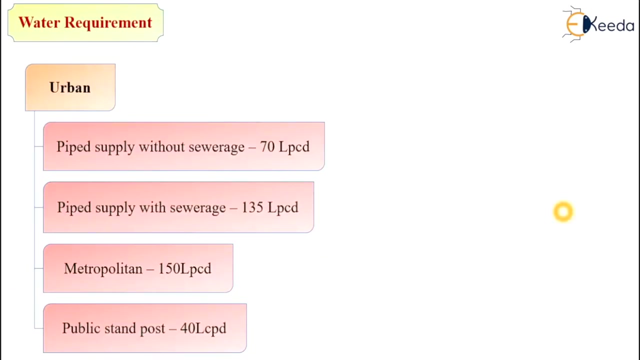 development program for cattle. So in rural area the basic requirement of water supply is greater than 40 L per capita per day and in addition to that we are considering the some extra water requirement or additional water requirement for the desert. In urban area, if the water distribution is through the pipe supply without sewerage, then 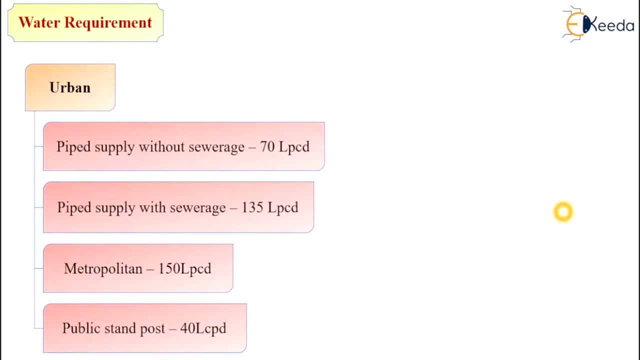 per capita requirement of water is 70 L per capita per day. if pipe supply with sewerage system are provided, then the water demand is 135 L per capita per day. in metropolitan city, again, this water demand is increased upto 150 L per capita per day. 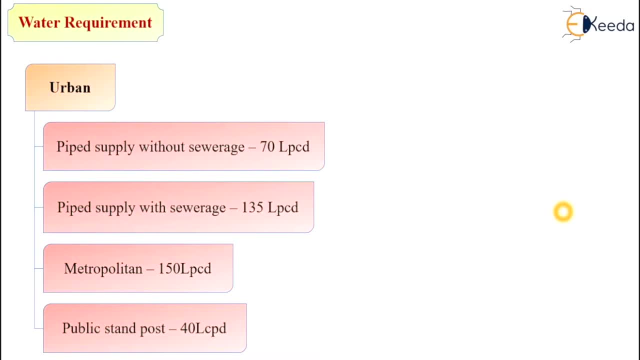 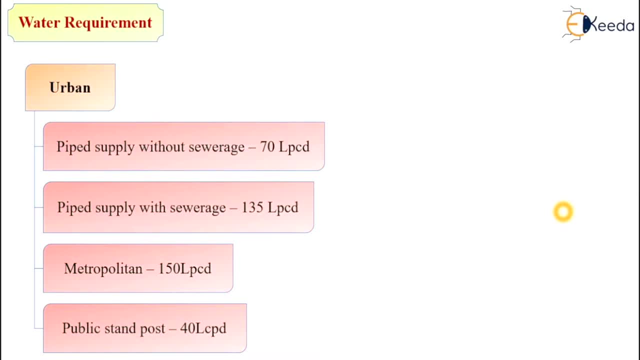 So for that one hand pump it has to beДаctor capital per day. Summon them down to the vertical feeling, and if the water supply is thicker in this case, then it should be less than 90 L per capita per day, and in public stand costs the requirement should be less. 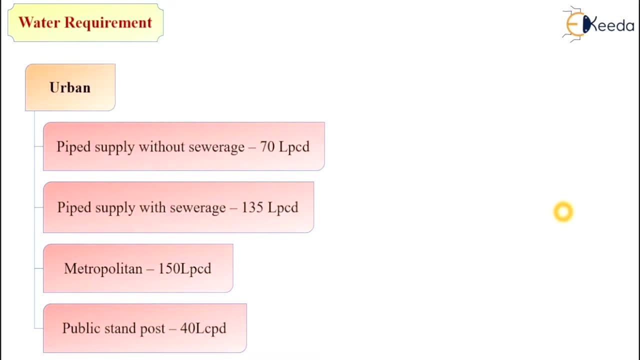 or reduced upto 40 L per capita per day. So these values of water supply requirement that are useful to calculating the total flow or design flow or design of sewerage system or design of any treatment plant, So these figures are very much important. generally in the urban area, the distribution system is: 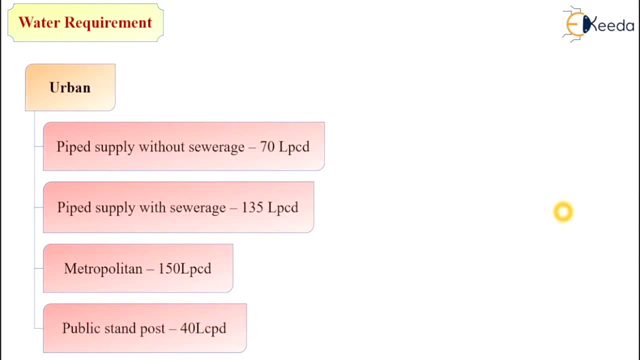 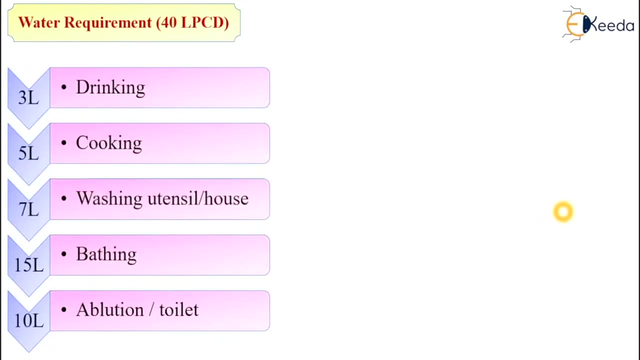 pipe supply with sewerage are provided. so generally, normally we are considering this figure, that is, 135 liter per capita per day. this is the water supply requirement or water demand. so this is the contribution of water requirement by considering the 40 liter per capita per day. 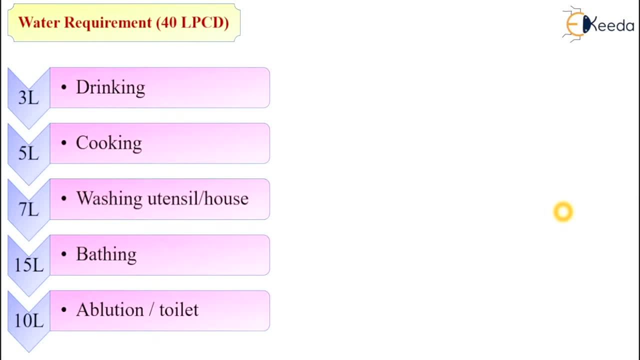 so this is the total use of water per day, which includes the water for drinking water, for cooking, water for washing utensil and house water for bathing and water for toilet. so combinedly all this usage, the figure is comes to 40 liter per capita per day. 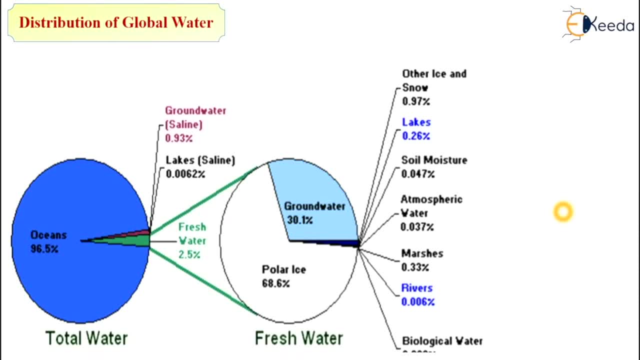 then this is the diagrammatic representation of distribution of global water, so as you can see in this blue circle the total water. out of this total water availability, the 96.5 percent water is available in ocean. then the remaining this 2.5 percent is the storage of fresh water. 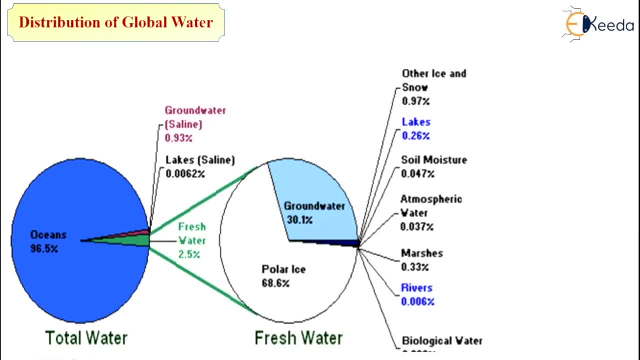 so again, fresh water includes the ground water and polarize, so groundwater, again, groundwater contribution is minimum and polarized contribution is maximum. so again some minor concentration or percentage, that is 0.0062, which is comes under lake or saline water, but generally that cell saline water or sea water. 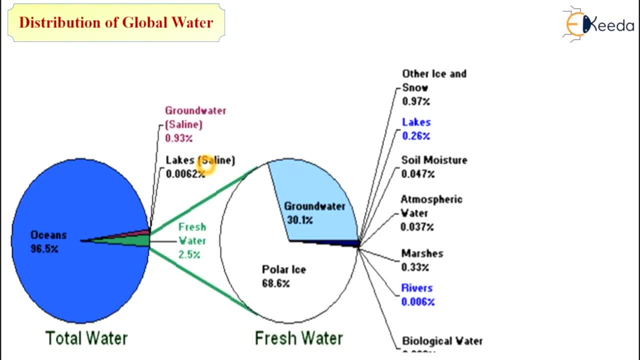 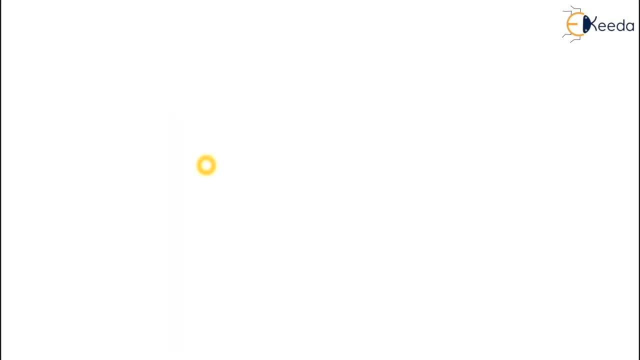 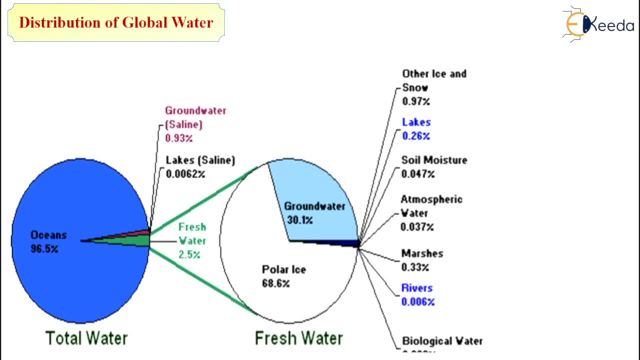 we cannot be used for the drinking purpose as it contains salt: 0.99 percent of saline water which is underground. so again because of salt content, we are not using this water for the drinking purpose. so only 2.5 percent storage is occupied by the fresh water. so again, it includes. 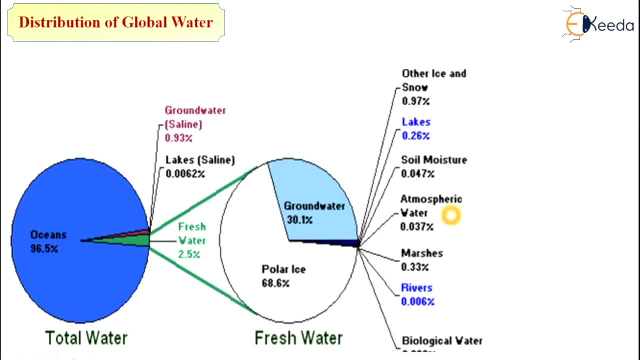 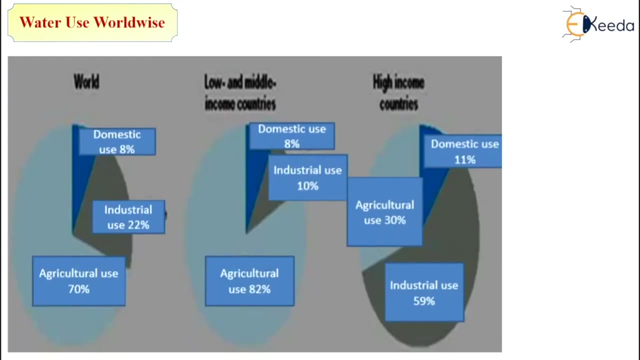 the lake storage, soil, moisture, atmospheric water, marshes, rivers and biological water supply. so this is the overall consumption of water, or storage of water, fresh water and ocean water. next, this is the chart of water usage of water worldwide. so, as you can see, if we are considering 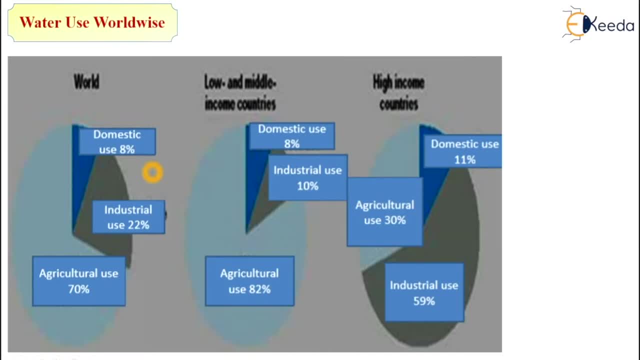 the worldwide consumption of water. the domestic use is 8 percent, industrial use is 22 percent and agricultural use is 70 percent. so maximum percentage of water is application, application for the agricultural purpose, low and medium income countries. the domestic or use is same, that is, eight percent. industrial is reduced up to 10 percent and agricultural use is maximum, that is. 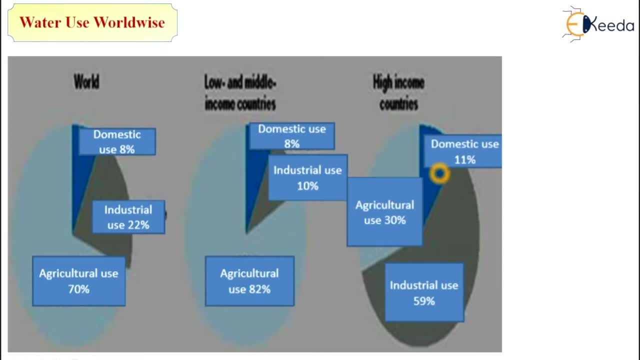 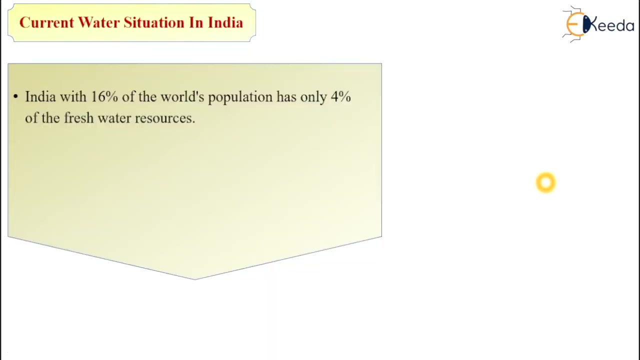 82 percent and in high income countries or metropolitan city domestic use is 11 percent, agricultural is 30 percent and industrial use is 60 percent because of the development of industrialization. so the industries: the water requirement for industrial activities is maximum in metropolitan or high income cities. so next is current water situation in india. india with 16. 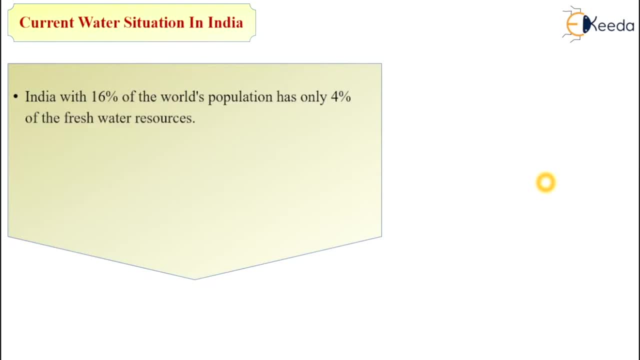 percent of world population has only four percent of fresh water resources. so the storage of fresh water- as we already seen in worldwide consumption of water use, it's very minor. so only four percent of out of 16 percent is considered as fresh water resources per capita. availability of fresh water in india. 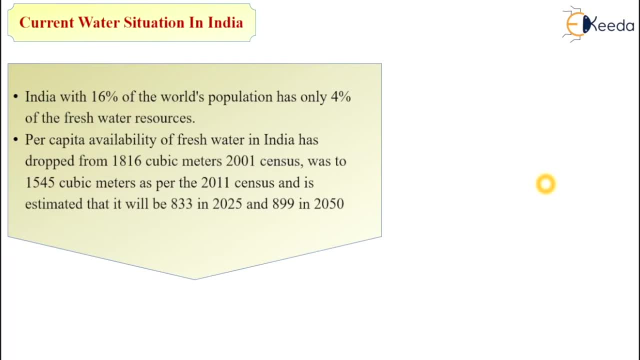 has dropped from 1816 cubic meter in 2001, was to 1545 cubic meter as in 2011 census and is estimated that it will be 833 in 2025 and 899 in 2050. that means the per capita availability of fresh water get reducing and 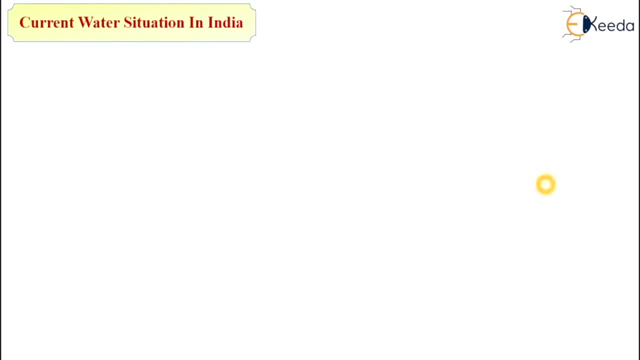 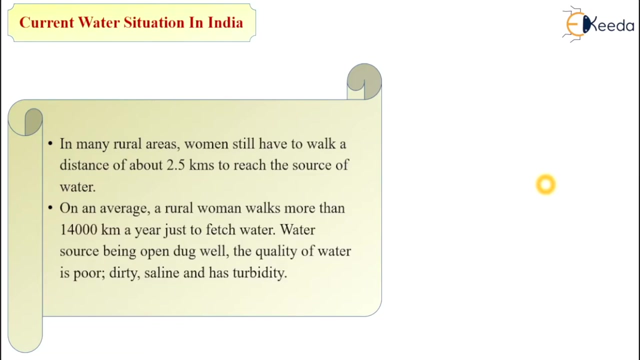 reducing again. in many rural areas, women still have to walk a distance of about 2.5 kilometers to reach the source of water. on an average, rural woman walk more than 14 000 kilometer a year just to fetch water. water source being opened up well, the quality of water is poor, dirty, saline and high turf has. 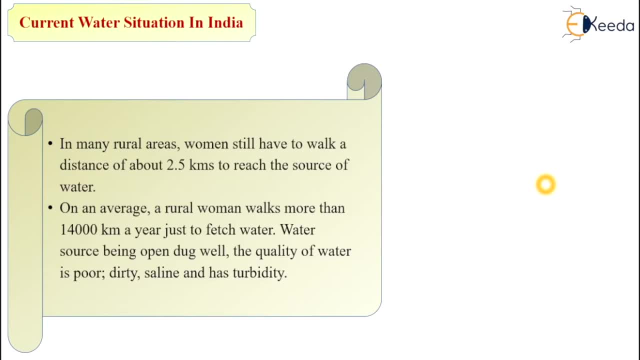 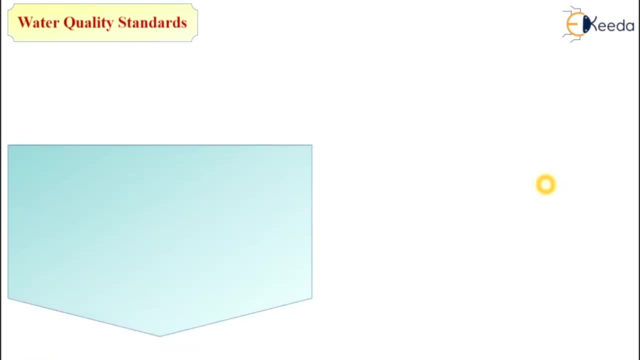 high turbidity. so in rural area there is again scarcity of water or there is inavailability of facilities of water supply or water piping systems. now to check the quality of water. as we have discussed, in rural, rural area the well water source is available for the drinking water purpose, but again the quality of that water is not good. 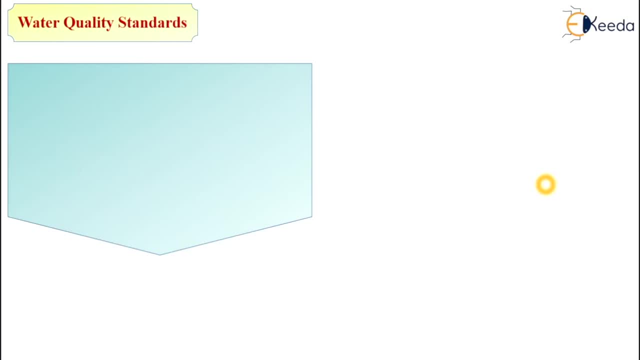 and in rural area there are facilities for treating water. treatment systems are not available in rural, rural acre, so that it is necessity to check its standards or permissible limit, or drinking is must now-a-days. so what is permissible limit? United States public health drinking water standards, that is, USPH, Indian. 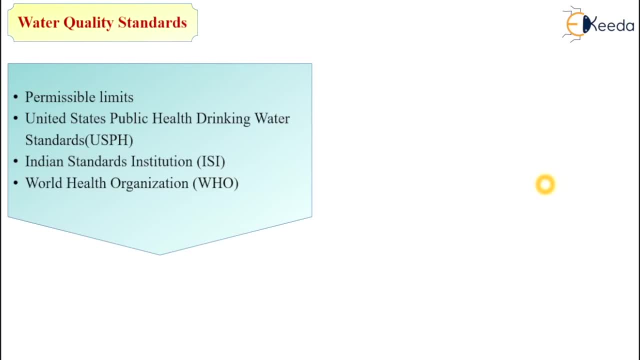 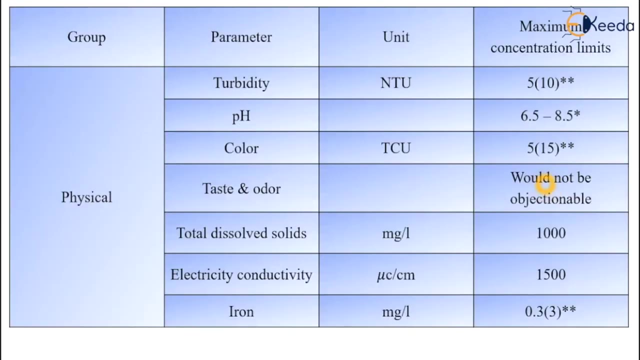 standard institution, that is ISR, and World Health Organization, that is FOO. so these three institutes are deciding the permissible limit or drinking water standards. so let's we see one by one. so these are the Indian standards of drinking water. so, as we have seen in previous lecture, the characteristics of 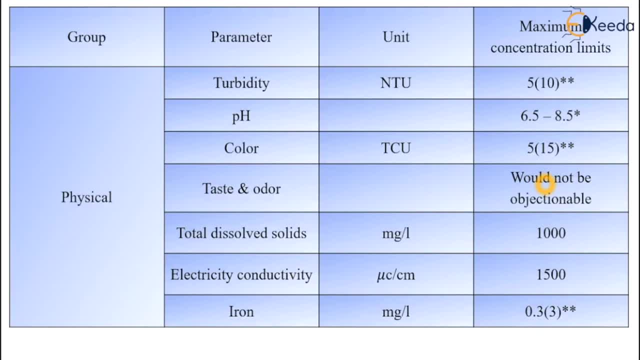 water in water quality. so there are physical, chemical and biological characteristics of water. under physical characteristics or physical parameters, there includes the turbidity, pH, color test and order, total dissolved solid, electricity, conductivity, ions, etc. so as you can see the units of each parameter and it's maximum concentration limit, that is, any. 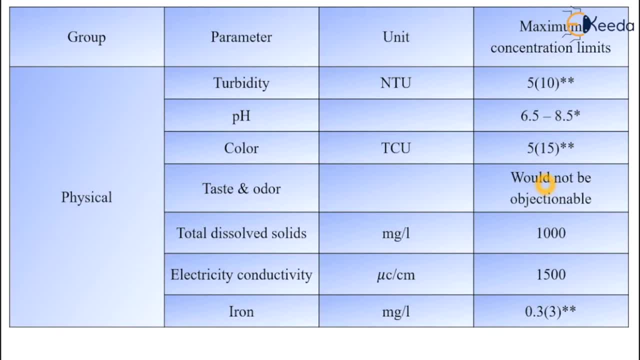 water source, for example river, lake, ocean, etc. which can be allowed the strain or characteristics or standards of water up to this limit, as may be known in this fourth column. so, for example, we have to check the turbidity of water in NTU. NTU is the unit of turbidity, that is neptelometer. 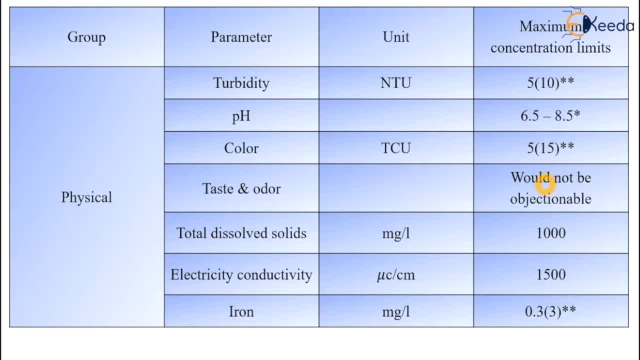 turbidity unit. so the maximum concentration limit is 5 and extended up to 10 that means more than 5 value the water which cannot be acceptable for drinking purpose. so for permissible limit, that is, maximum concentration of turbidity acceptable is 5. pH value is 6.5 to 8.5. there is no unit of pH. that is as 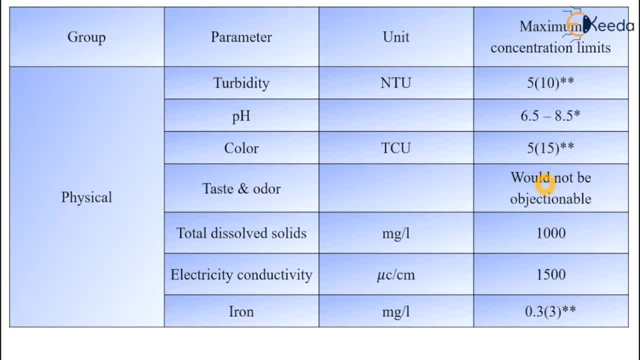 this also parameter we already seen in previous lecture. that is, if pH is less than 7, then water is considered as acidic, and if pH is greater than 7, then water is considered as alkaline. so for the drinking purpose the range should be 6.7. 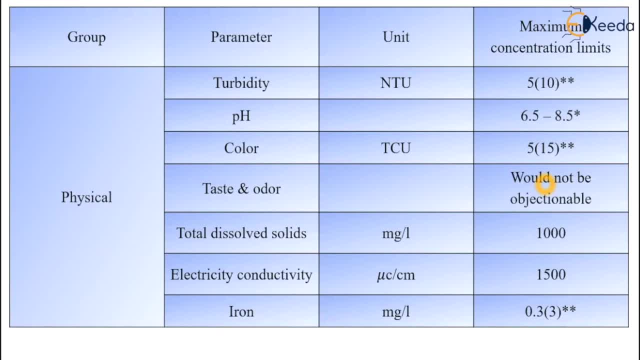 5 to 8.5. that means water should be neutral for drinking purpose. then color is up to 5 and extended up to 15, taste and order. the water would not be objectionable. would not be objectionable to drink and order. total dissolved solids: the maximum concentration limit is up to thousand electric and. 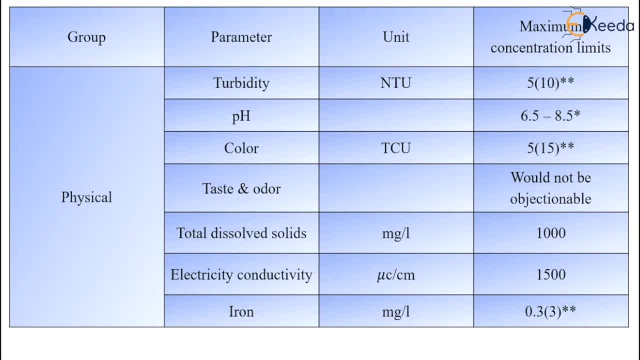 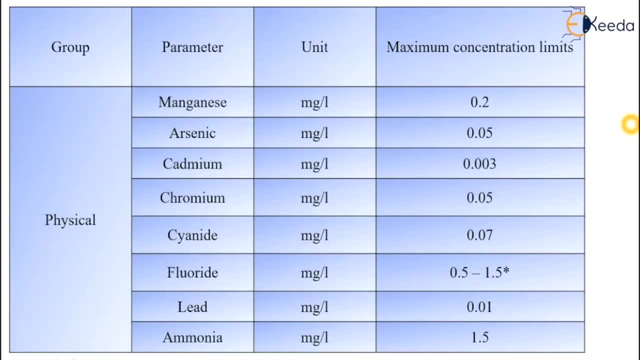 electricity conductivity is up to 1500 ions. contents are 0.3. thiscent inけれ bit of chlorine, CDTs value for the percent pressure charge. the Metallic Expandro Olein, Parents of the, gave again some trace elements that It is. it is the Blizzard Aqueduct, the 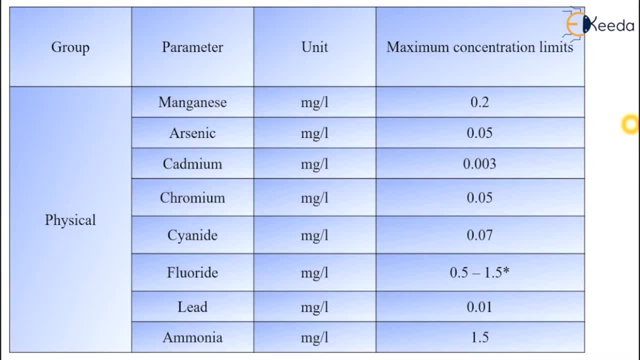 sam esseskádligé the istrinska medium: chromium, cyanide, fluoride, lead, ammonia, Etc. punch attack underneathесс gee. this trace elements are somewhat important for the body, human body, but I fact is to A respect is cut top pros and cons성, robust fuego ride picnic지만. you think are harmful for the human body. so if its concentration is exceeded, this is a for the human body. so it is max the amount of persona electric bone energy if because of the Ox, jinglewould filler peptide, if this is harmful for the human body, therefore these are harmful for the human body. so it'sBLE b있는 twoר. 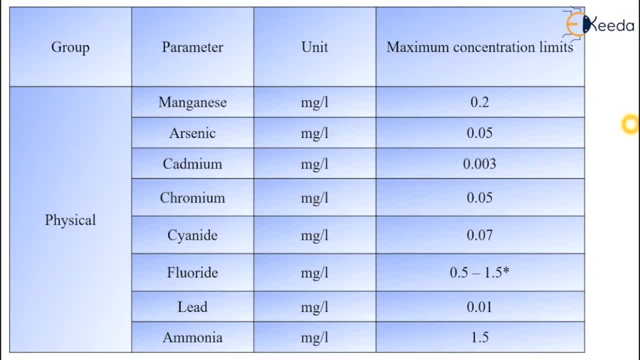 so its maximum concentration limit, as you can see in this column. so we cannot. if this concentration is exceeded, this water is harmful for purpose of drinking. so, as you can see, the manganese content is up to 0.2. arsenic is up to 0.05. cadmium is up to 0.003. chromium is up to 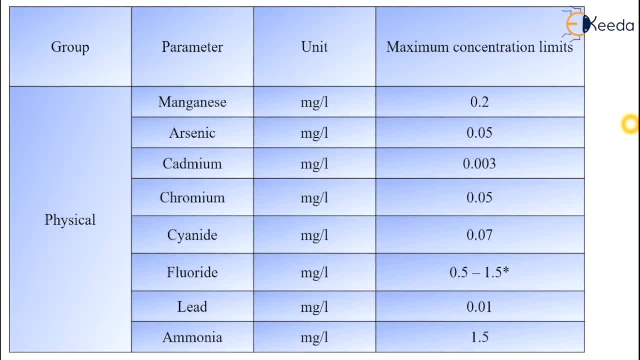 0.05, cyanide is up to 0.07, fluoride is up to 0.5 to 1.5, lead is up to 0.01 and ammonia is up to 1.5. the unit of these. all these parameters are in milligram per liter. 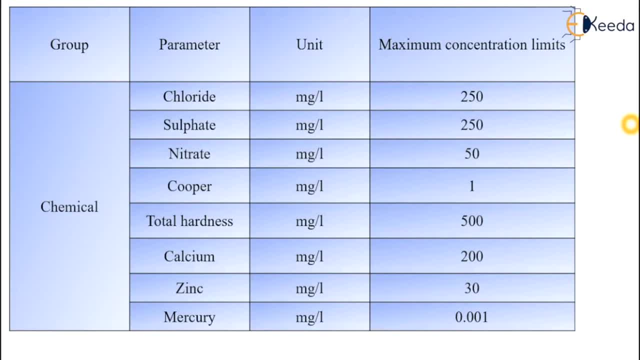 so next is chemical parameters. these also characteristics we already have seen. so under chemical parameters it includes chloride, sulfate, nitrogen, copper, total hardness, calcium, zinc, mercury. again, these parameters are essential for human body. but again its concentration is exceeded, then it will be harmful for the human. for the purpose of: 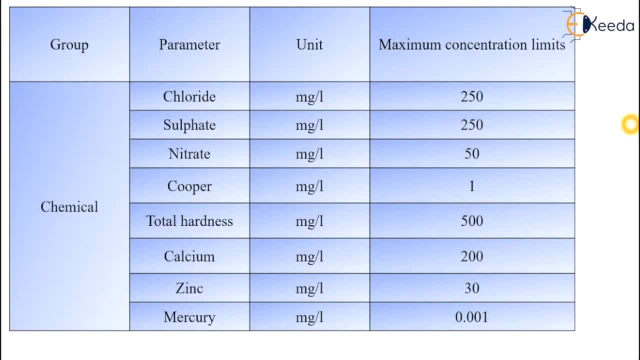 drinking water. so again, the chloride contains. the maximum concentration limit is 250. it is important parameter. sulfate content also similar to chloride, that is, 250 mg per liter. nitrate contents are 50 mg per liter. copper should be 1. total hardness should be 500 mg per liter. calcium should be 200 mg per liter zinc. 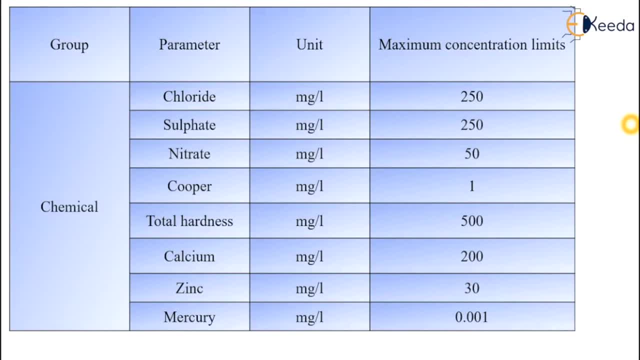 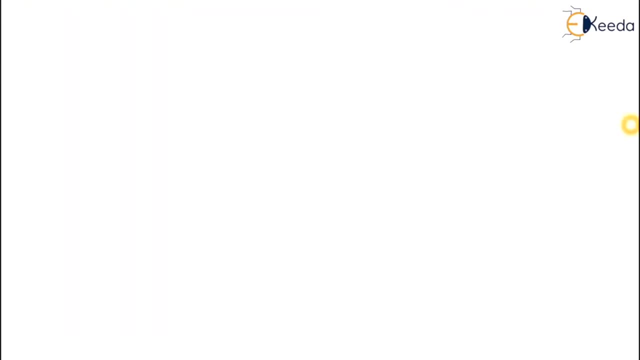 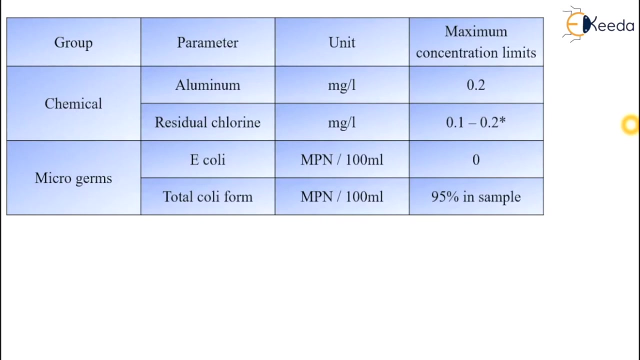 should be 30, and mercury. it is very harmful or toxic element for the human body when its concentration is exceeded of 0.001. so in very minute amount it should be present in water, but it is essential. then next is aluminium should be 0.2 milligram per liter and the residual chlorine should be 0.1 to 0.2 mg per liter. 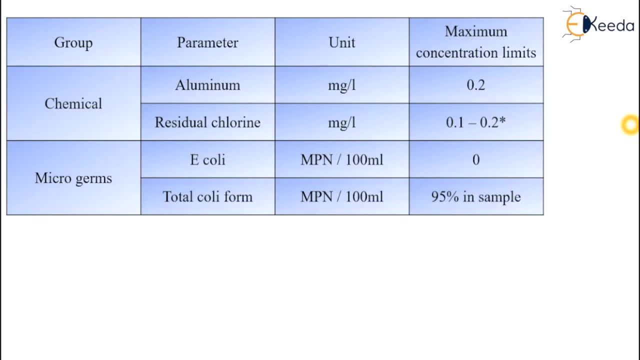 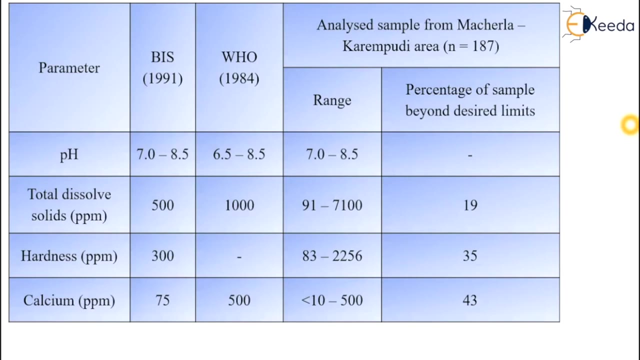 again under biological characteristics, the e coli, or germs, must be absent in drinking water. that should be nil or zero. so next, these are the again standards, or permissible limits, and, as you can see, this is the comparison or different values for the indian standards and for the world health organization. 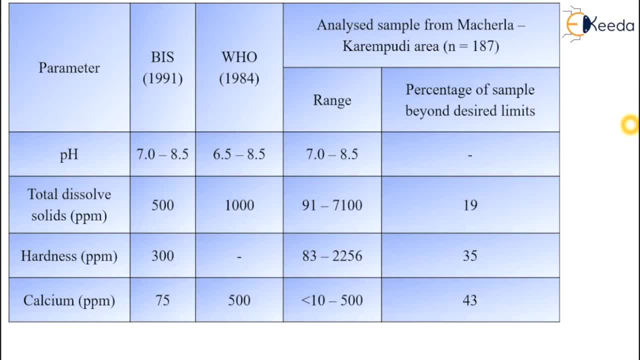 so there is not much difference in these two values. as you can see, the ph range is almost same. the total dissolved solids is in the range of 500 to 1000. hardnet should be 300, calcium should be 75 to 500. magnesium should be 30.. 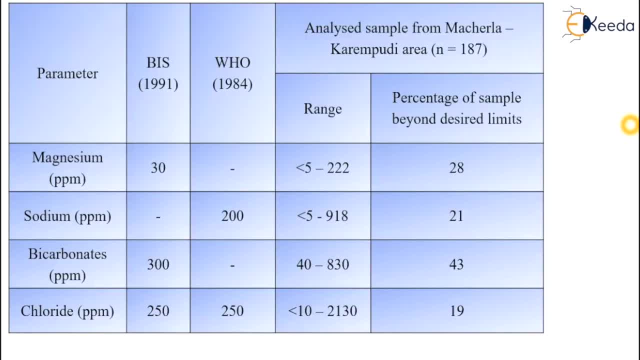 sodium should be 5 to 918. bicarbonate should be 30 mg per liter. chloride should be 250 mg per liter. so as you can see in this last column, these are the percentage of sample beyond desired limit. that means if this water exceed this values of parameters then it should be harmful for the 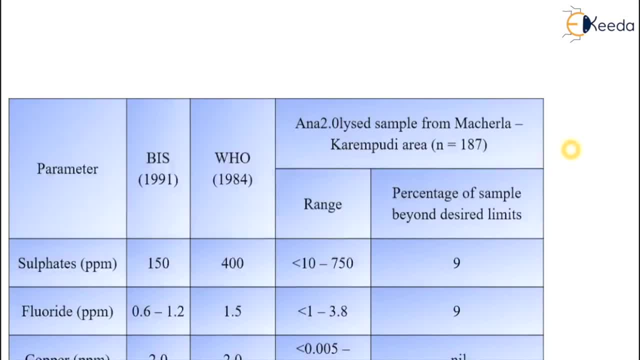 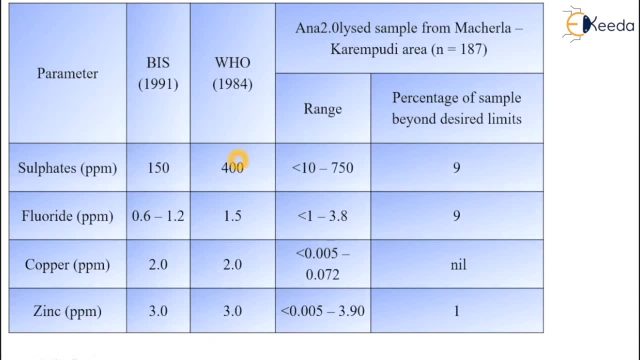 drinking purpose or we cannot drink this water again. sulfate contains: as per indian standard, the value should be 150. as per world health organization, the value should be 400.. fluid content up to 1.5. copper value is same for both the standards and zinc value also same for both the standards. so there is not much difference in. 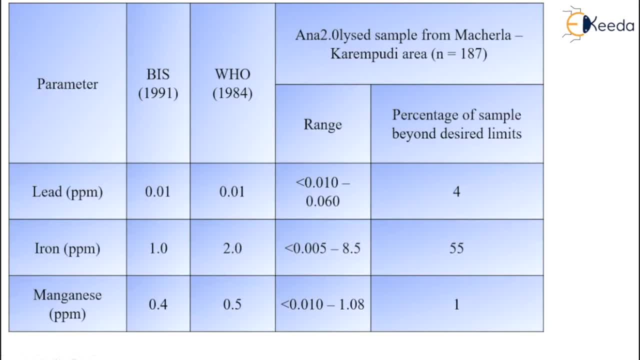 this tool. again, lead concentration is very minor, that is, 0.01. similar for both. the iron contents are one to two mg per liter and manganese content are 0.4 to 0.5 mg per liter, and the iron content is 1 to 2 mg per liter and the manganese content is 0.4 to 0.5 mg per liter. 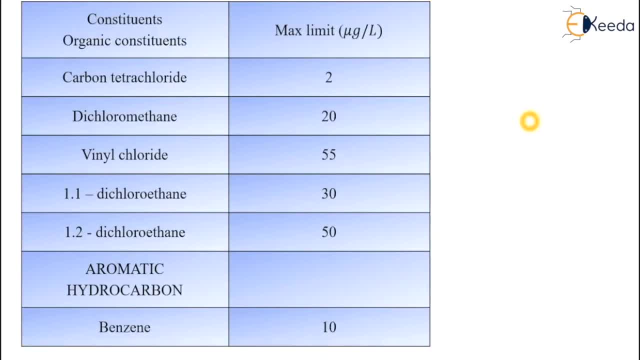 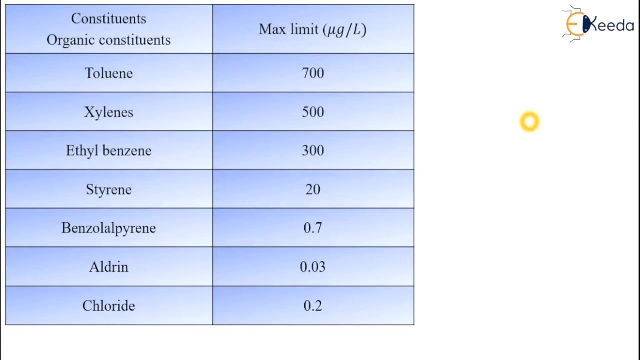 so, again, these elements are essential for body, but its concentration is exceeded its limit, then it will be harmful or we cannot drink this water again. next elements are toluene, xylene, ethyl benzene, ethyl benzene, stearine, i'll, aledrine chloride, etc. again, this concentration is minor, as you can see its values. 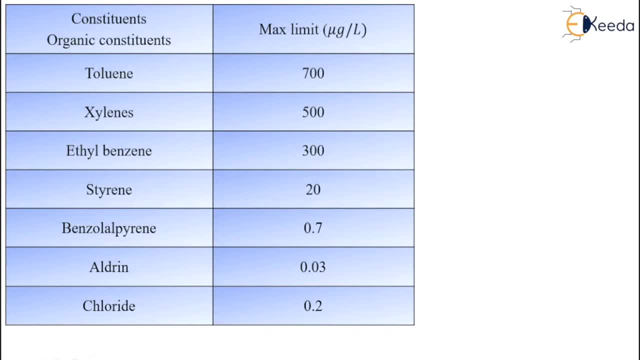 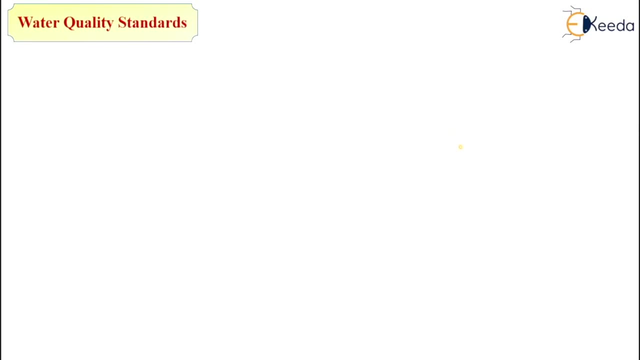 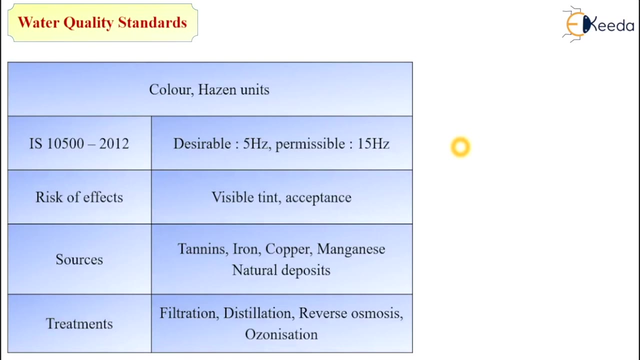 but if these values are exceeded to this limit then it will be harmful for drinking purpose or for human health. so next we will see the one by one water quality parameters, water quality standards for one by one parameter. so first are the physical parameters. so under physical parameters, the first 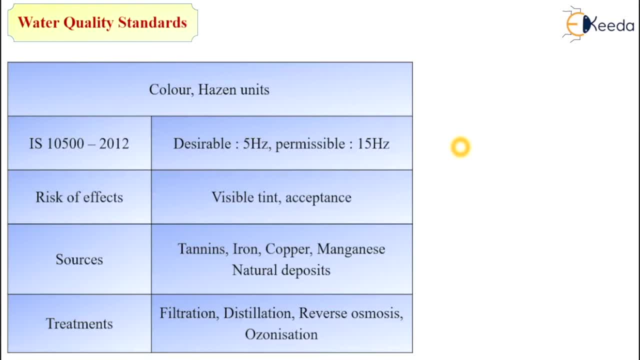 is color. so, as per indian standard, the desirable limit for color is phi, value is 5 and permissible limit is 15.. that means that water contents color value, color unit is 5, has an unit, then it should be drinkable, or we can drink this water, but its value, the permissible limit, is 15. that means 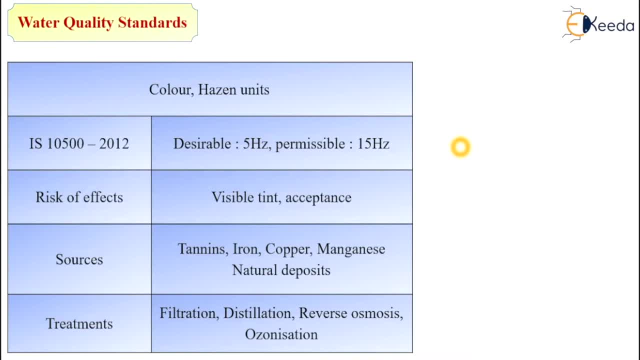 above 15 or higher, then formula should be recommended in standard class only. but it is not recommended in standard class of Keynesian 15 or greater than 15. that water is not acceptable for drinking purpose. The risk or effect: that means: if this value is exceeded by 15 then it is not acceptable. The sources of color. 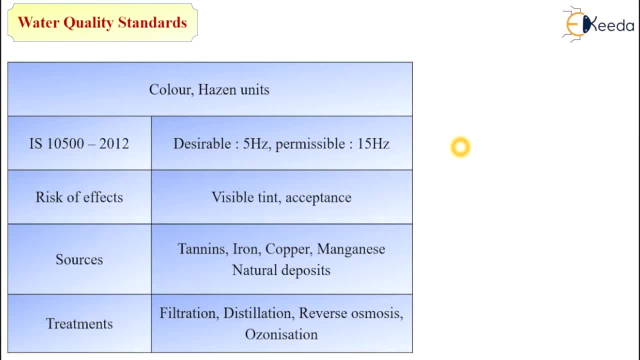 are tannins, ions, copper, manganese and natural deposits. Treatment to remove the color from drinking water are filtration, distillation, reverse osmosis and ozonation. So, as you can see, this is the color of water and we can remove it by this treatment. that is, filtration. 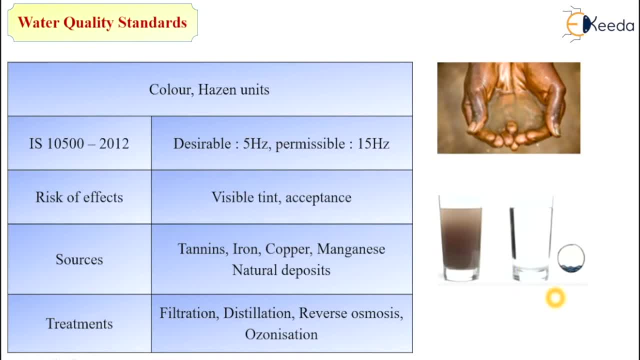 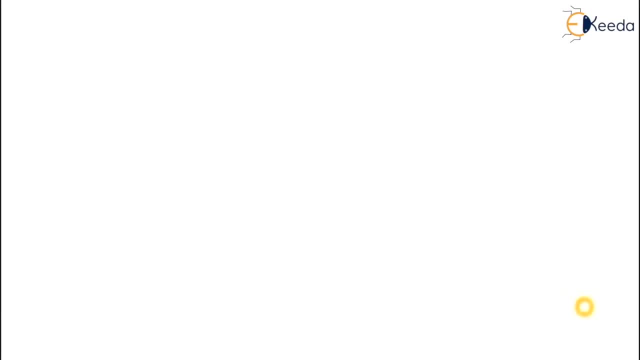 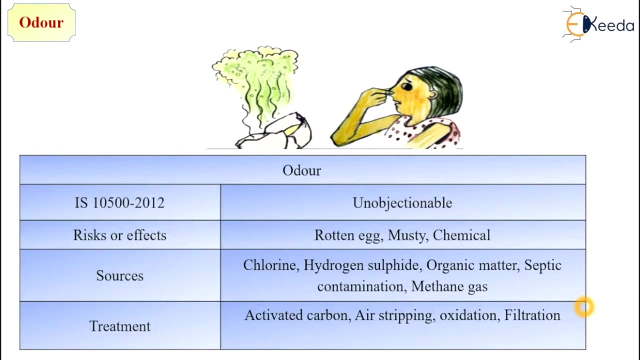 distillation, reverse osmosis, ozonation, etc. And, as you can see, the drinking water is always colorless. Next parameter is odor. As per Indian standard, the odor is unobjectionable. The risk or effect are rotten eggs, musky and 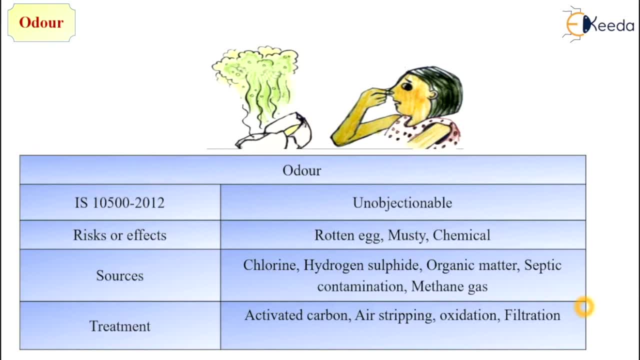 chemicals. Sources for consuming odor are chlorine, hydrogen, sulfide, organic matter, septic contamination, methane, gas, etc. The treatment to remove odor from water is activated carbon, airstripping, oxidation, filtration or some aerobic treatments. Next parameter is the water. As per Indian standard, the odor is unobjectionable. The risk 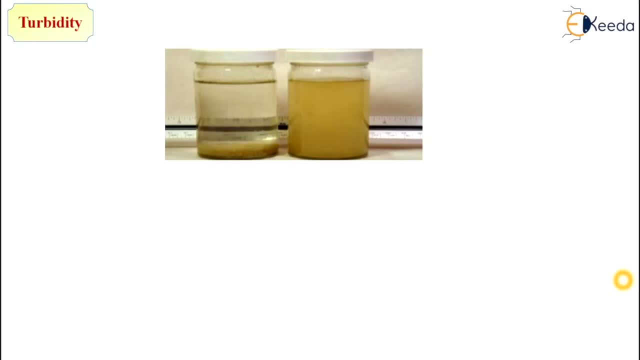 or effect are rotten eggs, musky and carbon. The treatment to remove odor is unobjectionable. Next parameter is the water. As per Indian standard, the odor is unobjectionable. The drink, or util d, is empty, but here it is the acid nucleate includin which helps in一下 dilution. 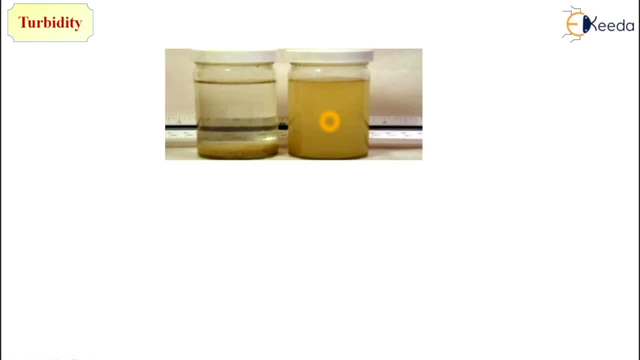 or filtration or depletion, and this is called purification of water. Next parameter is turbidity. As you can see in these figure, this is the turbid water and if this water is provided at sufficient prime, all the sediment particles or turbidity present, present in form of impurities, are settled down by the force of gravity and the clean water. 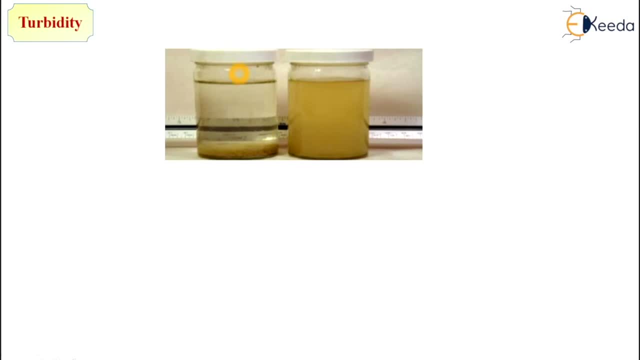 is taken from this above portion of this water. Next parameter is the air, Since the water from the sea- Benayan Turb, Judy- offer a salinity plateau on a liquid water level of heroin- This cannot defuse it- andty during freezing of water. 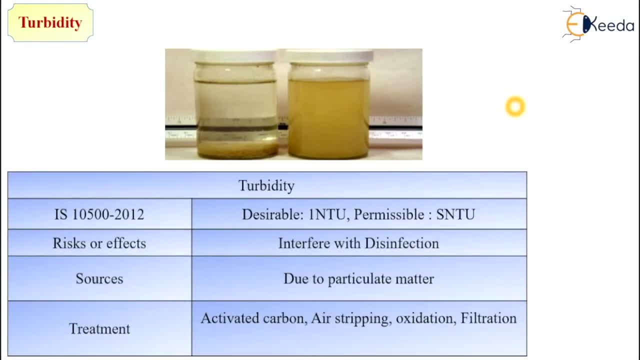 So as per Indian standard the desirable limit for turbidity is 1 NTU ie naphthalometric turbidity unit and permissible limit is not significant or 5 NTU ie. 1 to 5 range is acceptable, but above 5, the water is not acceptable for drinking. 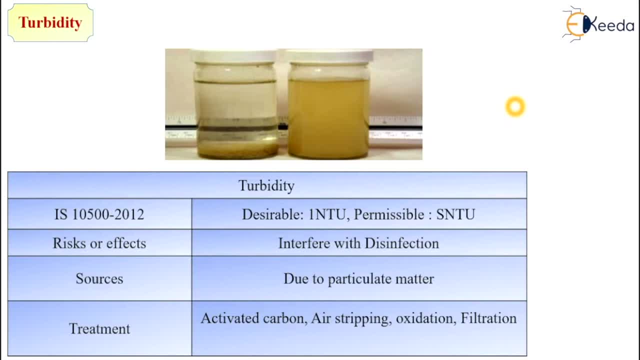 The risk or effects are it interfere with disinfection? That means if water is turbid, the disinfection process is not properly work out. The sources of turbidity are due to the particulate matters. The treatment should be provided to remove the turbidity is activated carbon, air stripping, oxidation and filtration. 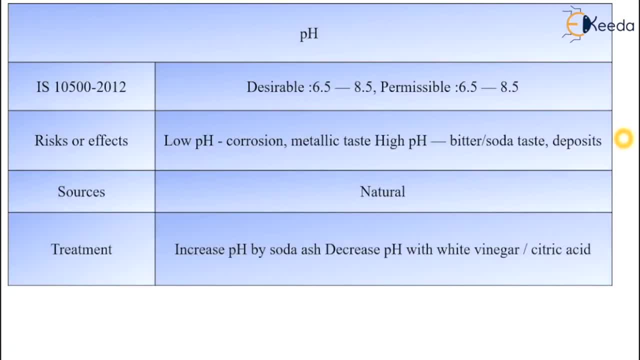 Next is pH. As per Indian standards, the desirable limit for pH is 6.5. If pH is low, the water is acidic in nature and it should be corrosion metallic test high. And if pH value is higher than 7, that means the water is alkaline in nature, So it imparts a bitter taste to the water and deposits in water. 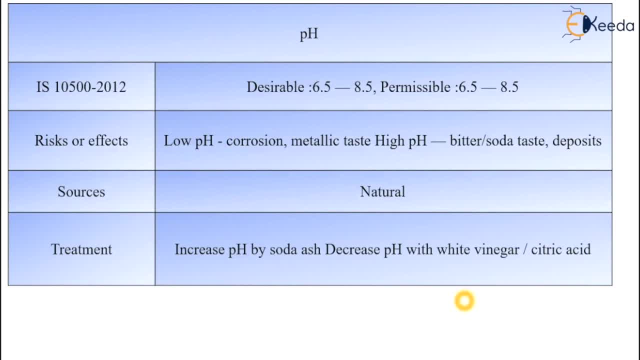 So to maintain the pH, we are increase the pH value. If the water is acidic in nature, then we are adding soda ash to increase its pH, and sometimes, for decreasing the pH value, we are adding the white vinegar or citric acid. 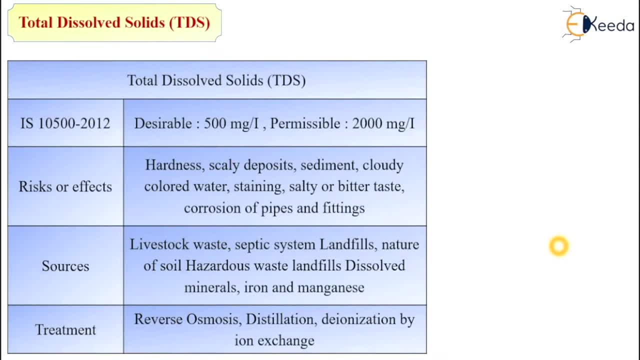 Next parameter is total dissolved solids, TDS. TDS are 500 MG per liter and the permissible limit is upto 2000.. That is the ranges in between 500 to 2000.. The risk or effect of total dissolved solid is it increases hardness, Scaly deposits are formed in this water, Sediments occur, cloudy coloured water, staining is there, salty or bitter taste is imparted to the water and corrosion of pipes takes place. 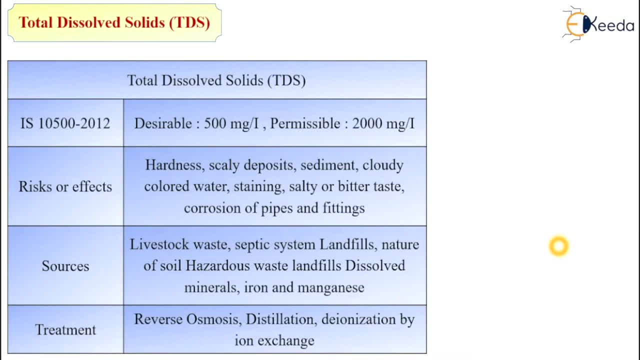 The sources of total dissolved solids are livestock waste, septic system landfills, nature of soil, hazardous waste landfills, dissolved minerals, ions and manganese, And treatment to reduce or to treat the water to remove. the total dissolved solids are in form of. 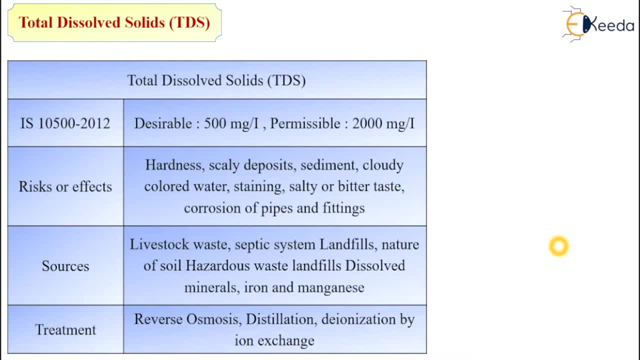 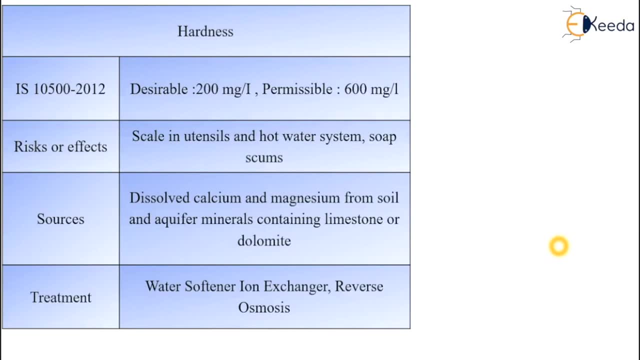 reverse osmosis, distillation, deionization or by ion exchange. Next important physical parameter is hardness. So as per Indian standard, the desirable limit is 200 mg per litre and permissible limit is 600 mg per litre. Risk or effect of hardness are scale in utensils and hot water system. soap consumption is maximum. 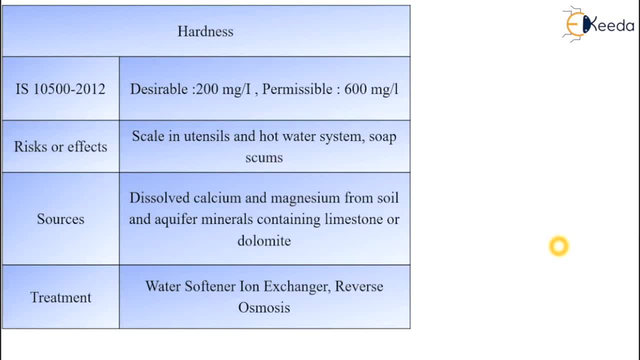 Sources of hardness are dissolved calcium and magnesium from soil and aquifer mineral containing the limestone or dolomite. So to treatment to remove the hardness are water softening such as ion exchange process or reverse osmosis. So all these treatments we are going to see in next lecture. 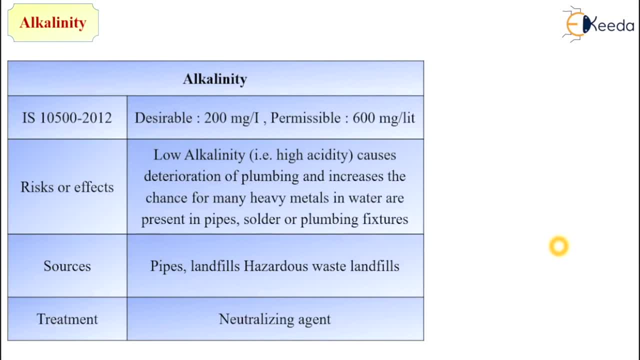 Next parameter is alkalinity. As per Indian standard, the desirable value for alkalinity is 200 and permissible limit is 600. The risk or effects are If low alkalinity- that means the high acidity- causes deterioration of plumbing and piping and increase the chance of many heavy metal in water- are present in pipe and plumbing fixtures. 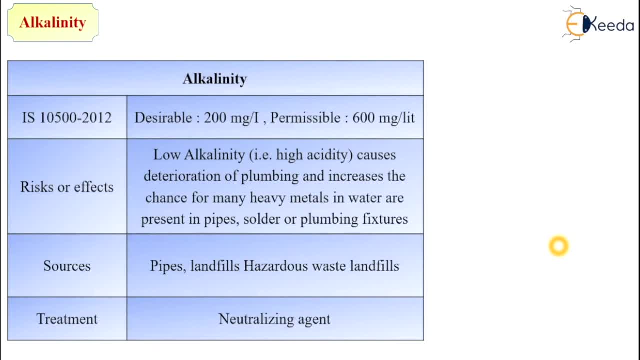 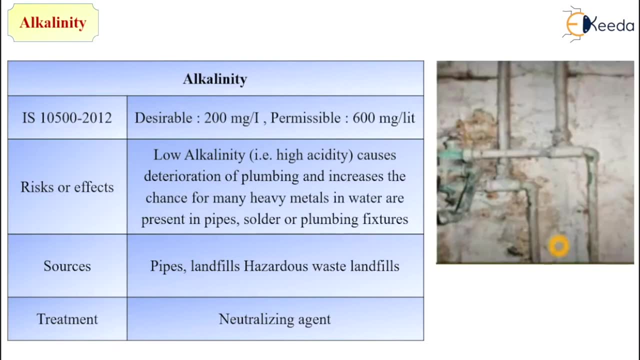 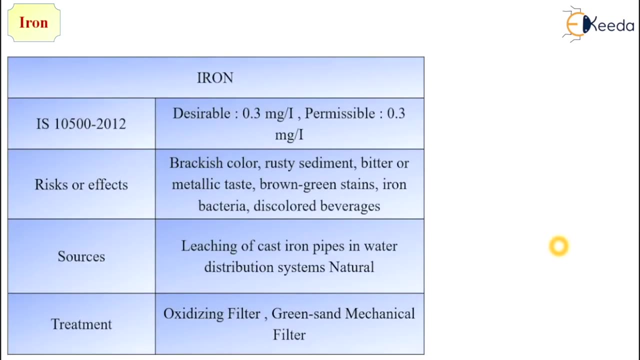 The sources of imparting alkalinity to water is pipes, landfills, hazardous waste of landfills. The treatments are Neutralizing agent, addition of neutralizing agents. Next are ions. As per Indian standards, the very minor quantity amount of ions should be present in water. 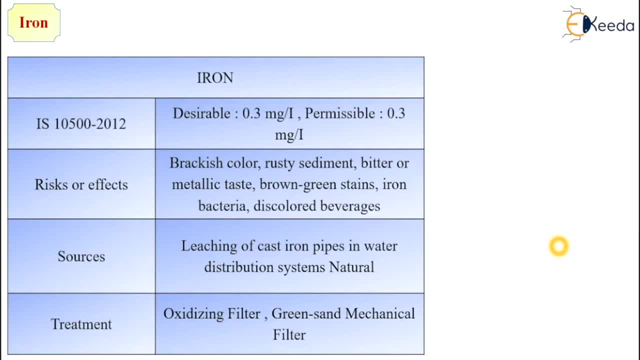 The desirable limit is 0.3 mg per litre and permissible limit also same, So it cannot exceed this value. So risk or effects for presence of ions above this value are: brackish colour is impart, rusty sediments, bitter or metallic taste, brown-green, stain, ion, bacteria discolour. 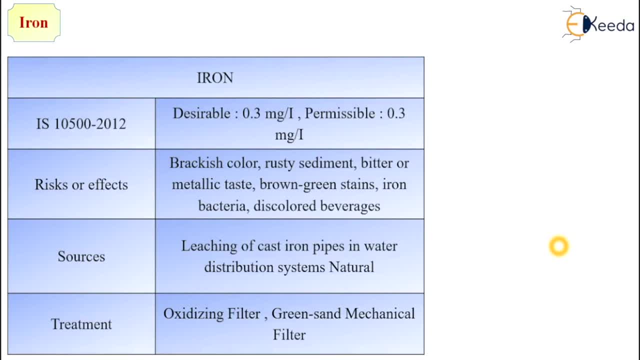 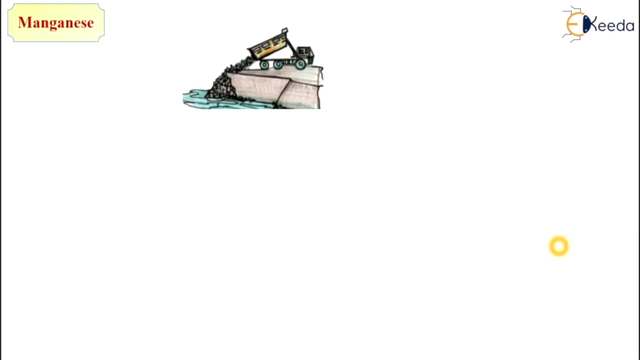 beverages, etc. The source of imparting ions in water are leaching of cast iron pipe in water and distribution system. naturally, The treatments provided for removing the ion contents are oxidizing filter, green sand, mechanical filter. Next is manganese. Again, the manganese contents as per Indian standards are: 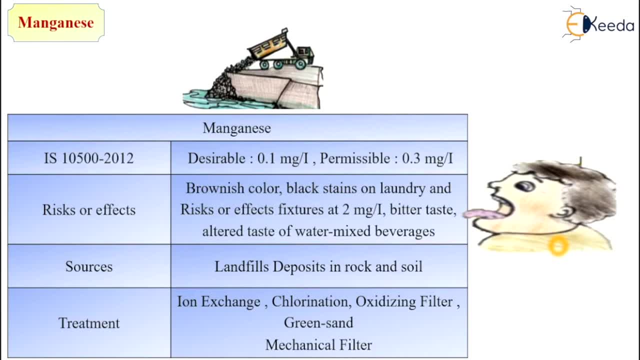 very small amount in water and in between the range of 0.1 to 0.3 mg per litre. So risk or effects are similar of ions content, ie Brownish colour, impart black stains on laundry- and risk or effect fixtures as 2 mg per litre. 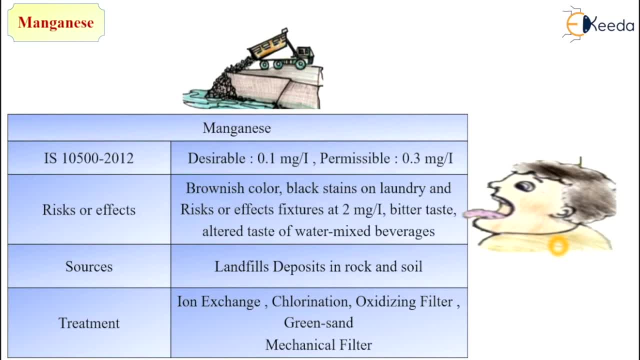 Bitter taste is impart and ultra taste of water makes beverages. The sources of content of manganese are Landfill deposits in rock and soil. The treatments provided should be in form of ion exchange, chlorination, oxidizing filter, green sand filter, mechanical filter, etc. 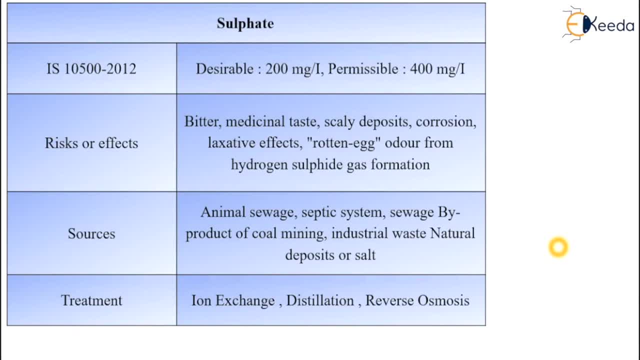 Next is sulphate. As per Indian standard, the desirable limit of sulphate is 200 and permissible limit is 400. The risk or effects are: The taste should be bitter, medicinal taste, scaly deposit, corrosion effect, rotten egg, odour from hydrogen sulphide and gas formation. 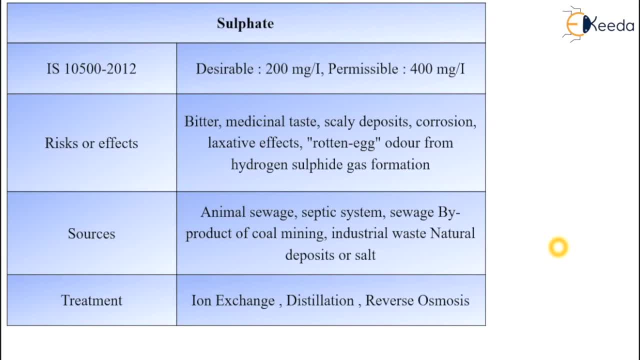 The sources are animal sewage, septic system, sewage by-product of coal mining, industrial waste, natural deposit or salt, And treatment should be provided in form of ion exchange, distillation and reverse osmosis. The next parameter is nitrate. 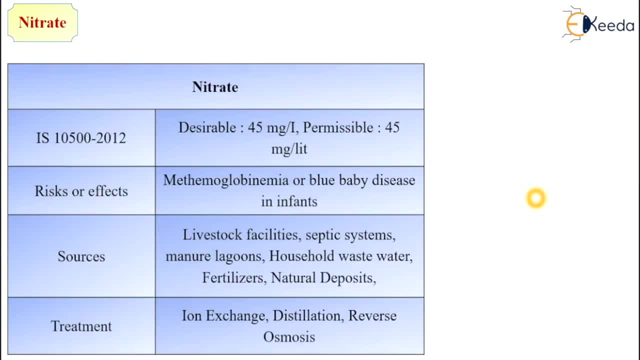 As per Indian standard, the desirable limit for nitrate is 45 mg per litre and permissible limit is same, ie 40 mg per litre. As per Indian standard, the desirable limit for nitrate is 45 mg per litre and permissible limit is same, ie 40 mg per litre. 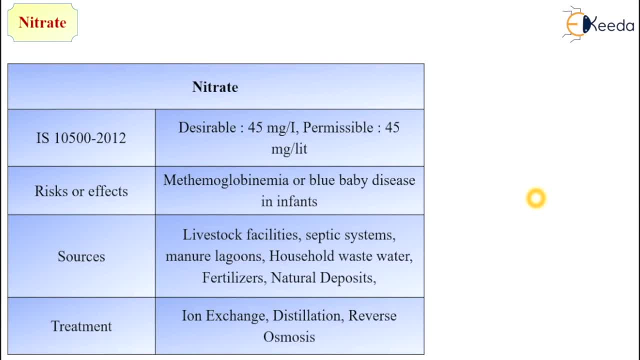 As per Indian standard, the desirable limit for nitrate is 45 mg per litre and permissible limit is same, ie 40 mg per litre. The risk or effects are The methyloglobinia disease or blue baby disease in infants. That means if nitrate content is greater than or exceed the value of permissible limit, then its disease is happening in babies. 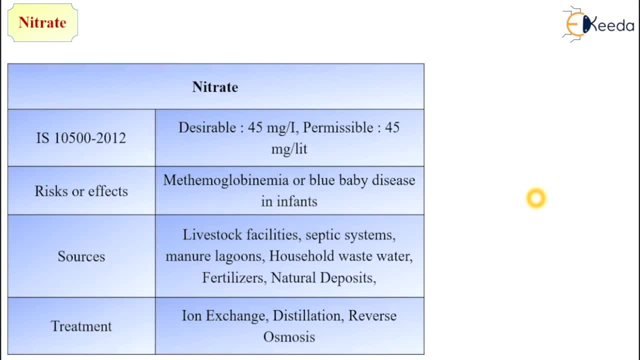 The sources of contaminant of nitrates contents are Livestock facilities, septic system, septic system, manure lagoons, household waste water, fertilizers, natural deposit, etc. And treatment to remove this nitrate contents from water are ion exchange, distillation, reverse osmosis. 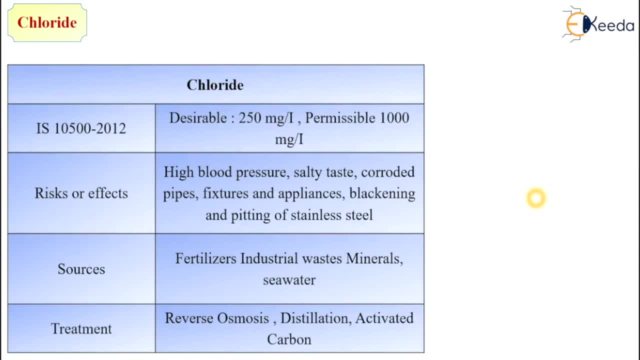 Next parameter is chloride. As per Indian standard, the desirable limit is 250 mg per litre and permissible limit is upto 1000 mg per litre. That means the value of 2000 mg per litre content in water. that water is acceptable for treatment. 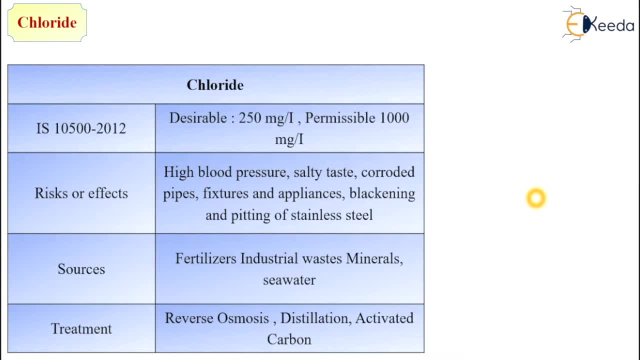 That water is acceptable for drinking purpose, but not exceeded this 1000 mg per litre. The risk or effects are High blood pressure, salty taste, corroded pipes, fixtures and appliances, blackening and pitting of stainless steel. Sources of chlorides are fertilizer, industrial based minerals, discharge into the water source or sea water. 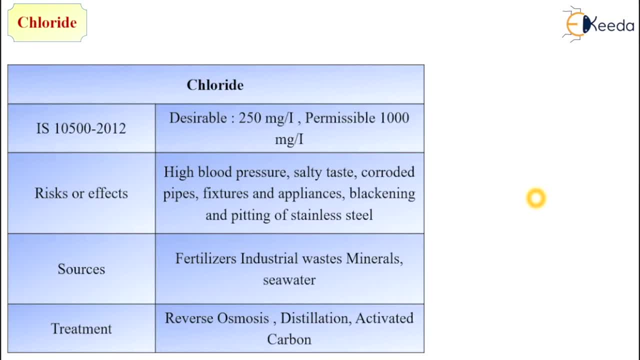 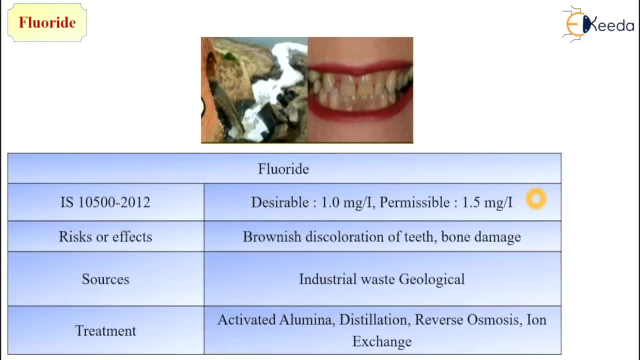 And treatments are provided to remove the chloride contents are: reverse osmosis, distillation, activated carbon. Next is fluoride. As you all of know, the exceeded limit of fluoride contains the fluorosis disease for the dental areas. So the desirable limit for fluoride is 1 mg per litre and permissible limit should be 1.5 mg per litre. not exceeded that 1.5. 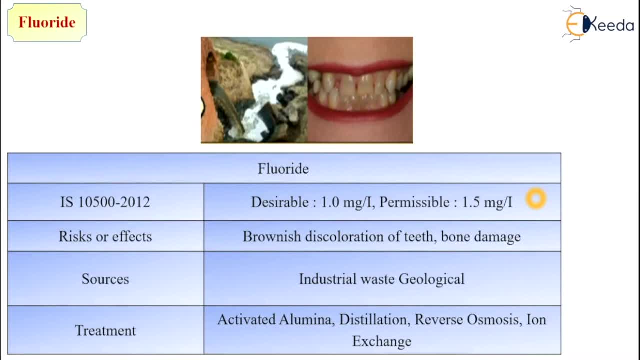 Risk or effects are Brownish discolourization of fluoride, Discolourization of teeth and bone damage. Sources are industrial based and geological water. Water contained in geological strata And treatments to remove fluoride contents are activated alumina, distillations reverse osmosis and ion exchange. 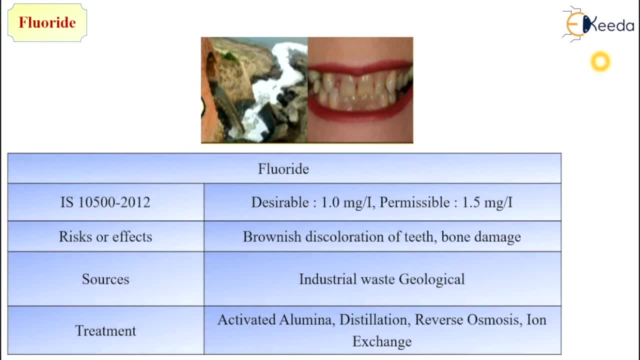 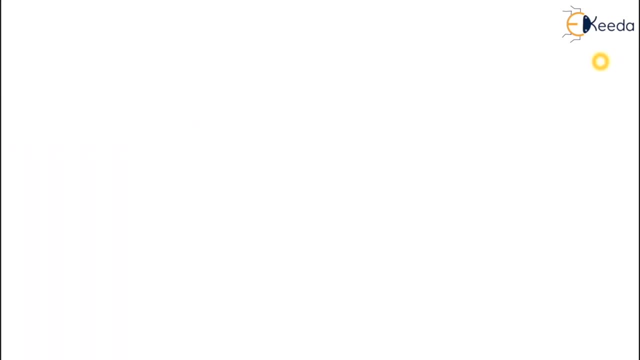 So most of the cation and anion form of fluoride contains, or ion contains, manganese contains carbonates, bicarbonates or fluoride contains nitrates, etc. Removed by the membrane technology that is, ion exchange, desalination and reverse osmosis processes. 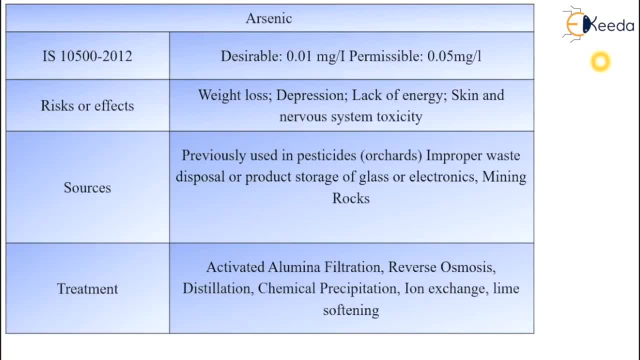 So that processes act as a advanced tertiary treatment that we are going to see in next lecture. The next compound is parameter is arsenic. The desirable limit for arsenic is 0.01 and permissible limit is 0.05.. The risk or effects are weight losses, depressions, lack of energy, skin and nervous system toxicity. 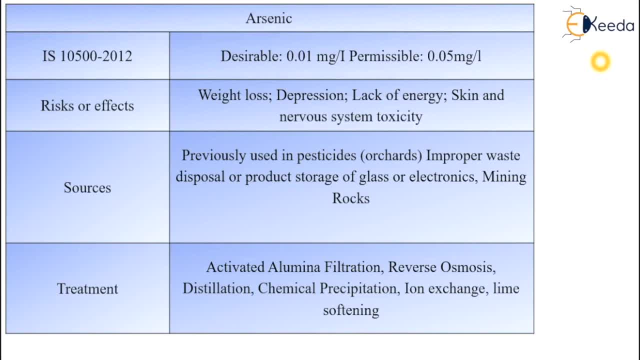 And sources are previously used in pesticides, improper waste disposal or product storage of glass or electronics. mining rods And treatments are provided to remove the arsenic contents are activated alumina filtration, reverse osmosis, distillation, chemical precipitation, ion exchange and light softening. 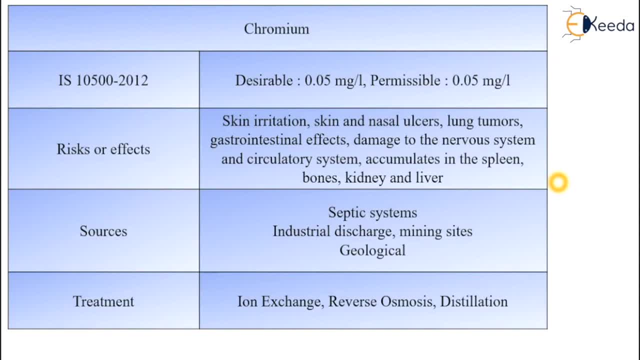 Next parameter is chromium. As per Indian standard, the desirable limit for chromium is 0.05 and permissible limit is 0.05.. So both the limits are same. So if we are exceeding this limit, then risk and effects are in form of skin irritation, skin and nasal allergies, lungs tumours, gastrointestinal effect, damage to the nervous system and circulatory system accumulated in spleen, spine, bones, kidney and liver. 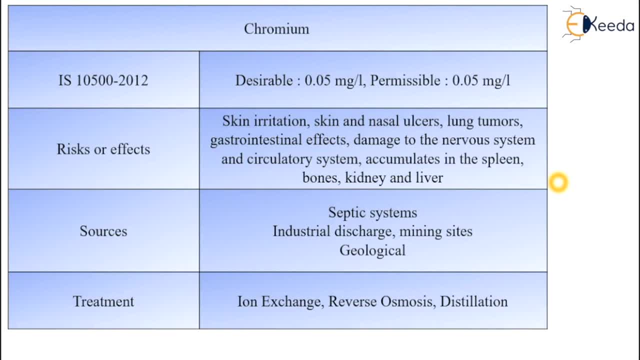 So it will affect to your directly to kidney. So this parameter is very much dangerous if its amount is exceeded beyond its limit. So it is desirable or permissible limit. Sources of generation of chromium contents are from septic system, industrial discharge, mining sites, geological sites, etc. 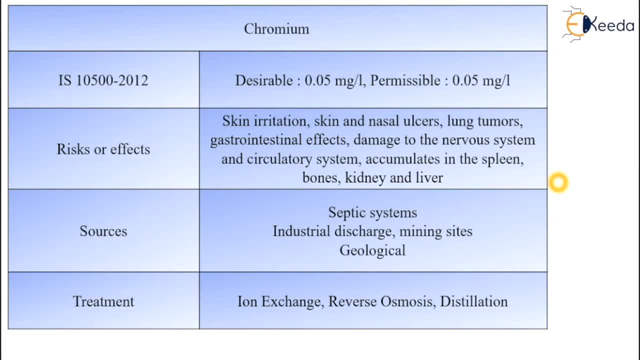 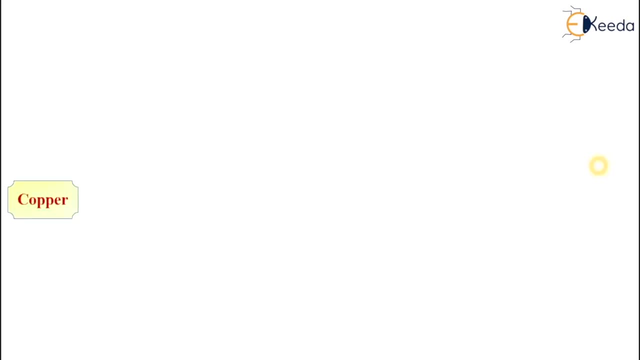 And treatment to remove chromium from the water or waste water are processes, again similar to the previous process which we have given to the cyanides removal or lead removal, That are, the ion exchange method, reverse osmosis and distillation methods. Next is copper. 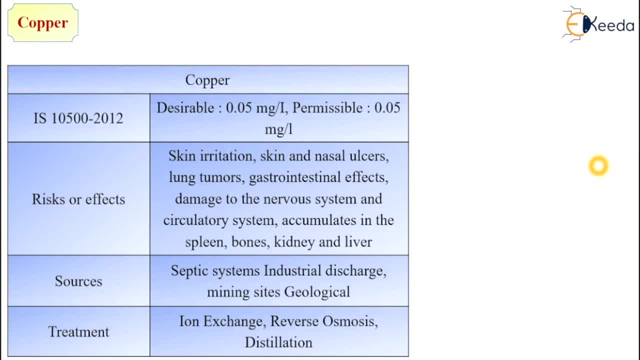 Again some amount of copper or some percentage of copper in water that are useful to the body, but again its limit exceeded its permissible limit. Then the risk and effects are applied to the human body in form of skin irritation, skin and nasal that similar to the chromium content. 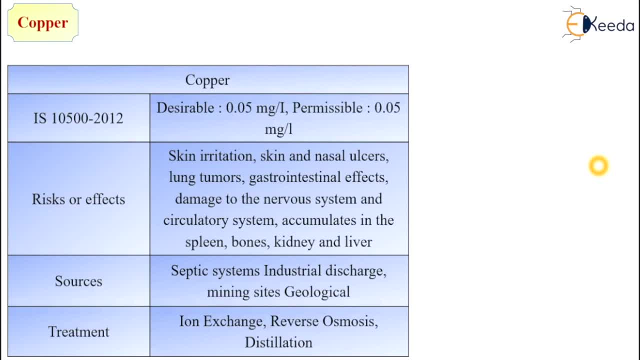 The similar effect, similar to the when the permissible limit is exceeded, as similar to the chromium content. So again, sources for copper generation are similar to the chromium content that are from the septic system, industrial discharge, mining sites and geological sites. And treatments are also similar to the chromium treatment, that are ion exchange, reverse osmosis, distillation and other membrane technologies, etc. 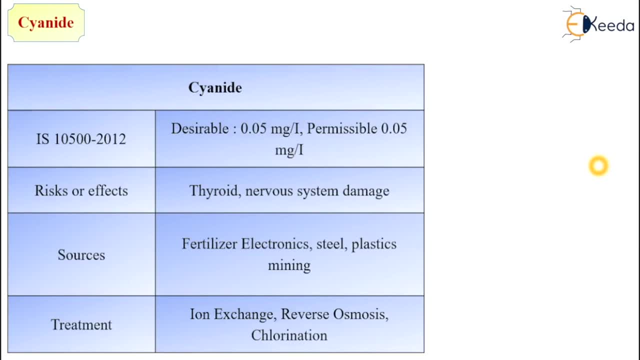 Next parameter is cyanide. As per Indian standard, the desirable and permissible limit of cyanide is 0.05.. So, as you observe that the chromium, cyanide and lead content are the value of that desirable and permissible limit are same, The risk or effect of cyanide contents, if exceeded, are it directly affect to the thyroid nervous system and damage the nervous system? 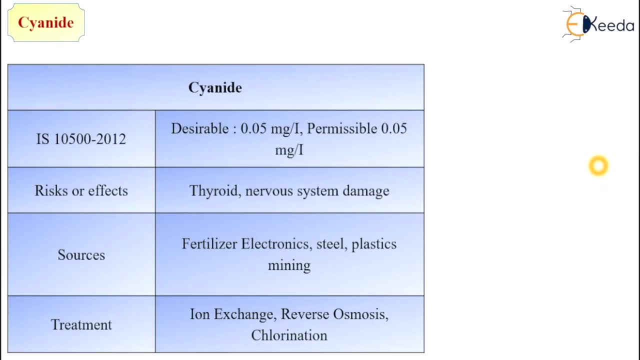 And sources of generation of this cyanide contents in water are from fertilizer, electronics materials, steel, plastics, mining, etc. And treatments provided to remove the cyanide contents or heavy metal from the water are ion exchange, reverse osmosis and chlorination. that is, disinfection. 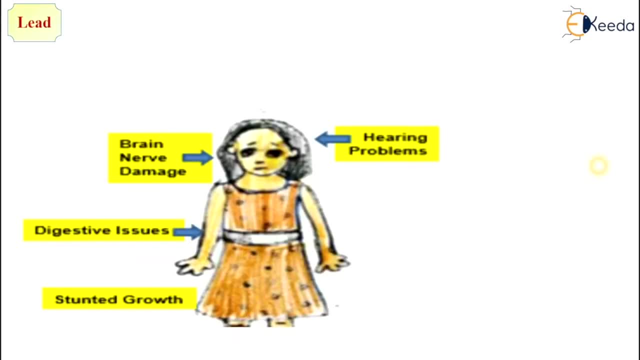 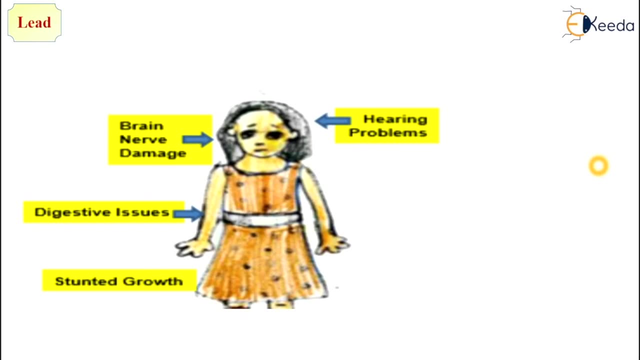 Next is lead. Lead is a very dangerous element when its amount is exceeded by its permissible limit. So it will directly affect to your nervous system, damage your nervous system. If you are facing some problems of hearing, then it will affect to your digestive system. 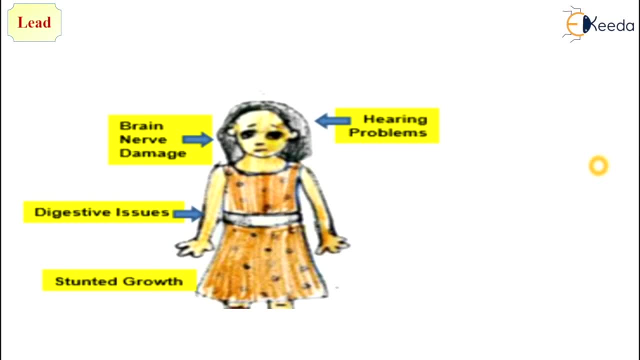 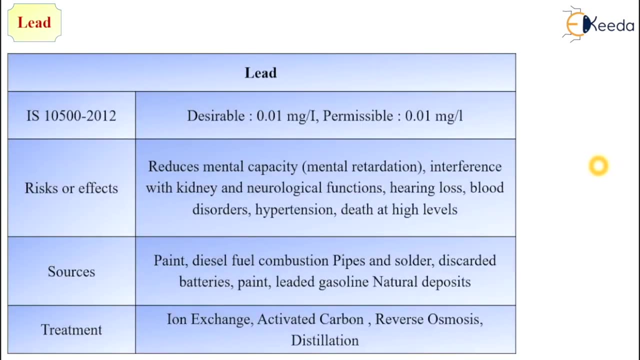 And also it will reduce the growth of human being. So as per Indian standard, the desirable and permissible limit of lead is very minute, that is, 0.01.. Risk and effects: when the lead content exceeded are: it reduces the mental capacity, That is, it will directly affect to your nervous system. 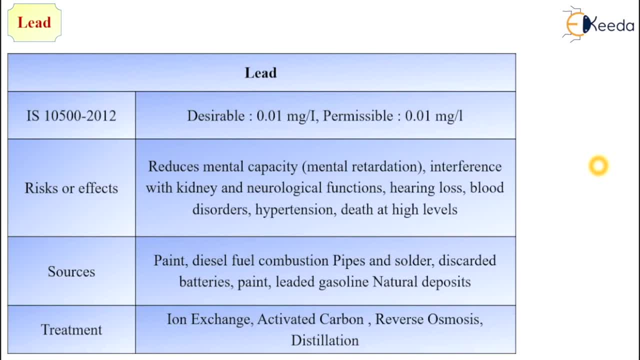 That it interfere with the kidney and neurological functions. Hearing losses are there, blood disordered hypertension is there, sometimes death at high levels. So sources of generation of leads are paint, diesel fuel, combustion pipe and soldiers, discarders, batteries, paints, other and other hardware which contains the lead. 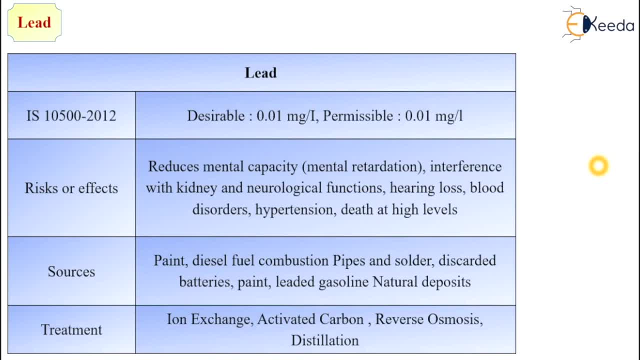 And when we are disposing this solid waste or directly into the ground, So it will not digested because of these are heavy metals So, and its burning is also dangerous. So the leachate formation from this or heavy metals are very dangerous And if it will infiltrated into the groundwater and many rural areas, they are using a groundwater for a drinking water source. 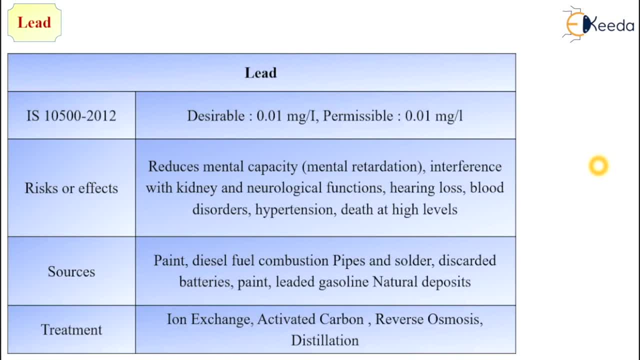 Then that groundwater if contain the lead which has the concentration exceeded its permissible limit, Then it will very dangerous And directly affect to your overall body system. So treatment to removing the lead are ion exchange, activated carbon, reverse osmosis, distillation, etc. 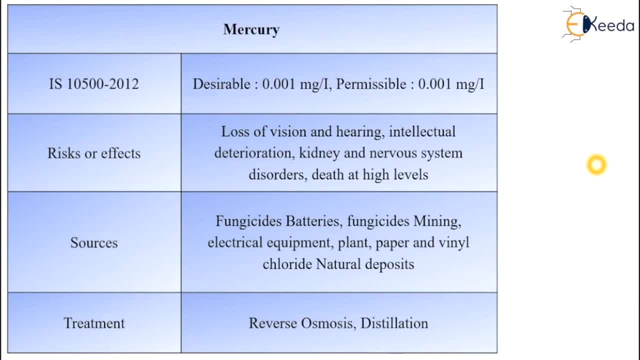 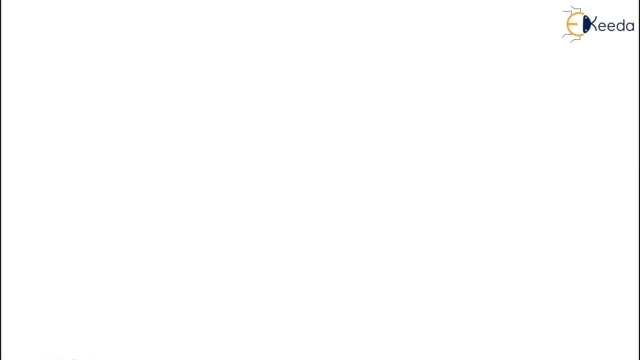 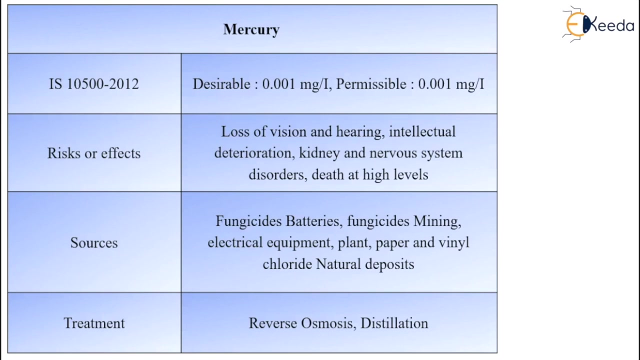 Next is mercury. As per Indian standard, a desirable and permissible limit of mercury that is 0.001.. Again, this amount is very minor. So risk or effects when this amount is exceeded beyond this permissible limit are in form of Loss of vision and hearing, intellectual deterioration, kidney and nervous system disorder, death at high level. 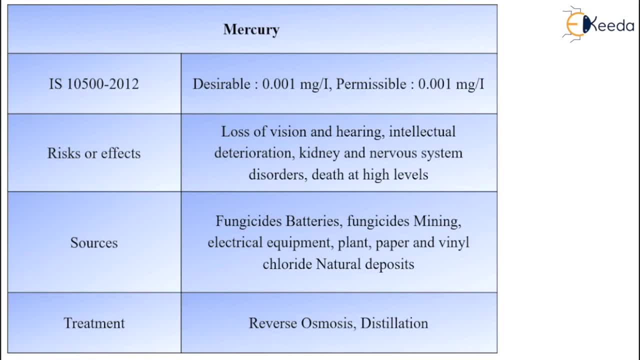 Sources of generation of mercury are from Fungicides, batteries, mining electrical equipments, plant paper and vinyl chloride paper industries, vinyl chloride natural deposits, etc. The treatments provided for the mercury remover are reverse osmosis and distillation. 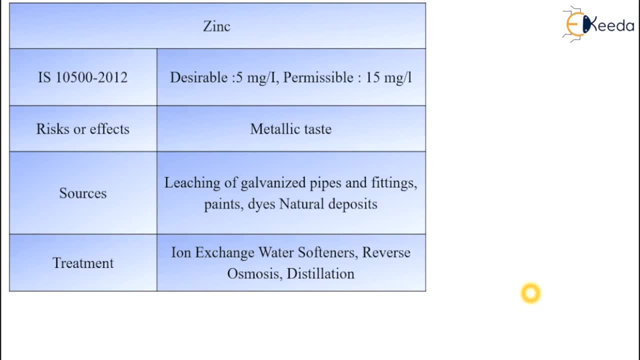 Next parameter is zinc. Again, zinc is very much important for body, but its desirable and permissible limit is 5 mg per liter And permissible limit is 15 mg per liter. That means if its quantity is exceeded up to the 15 mg per liter, then it will be acceptable for human body. 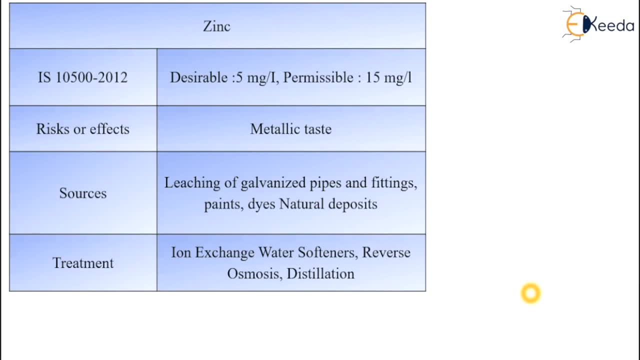 But If its value is exceeded beyond its permissible limit, then the risk are the metallic test. So we cannot drink this water as its test is in metallic nature. The sources of generation of zinc contents are from leaching of galvanized pipes and fittings, paints, dyes, natural deposits, etc. 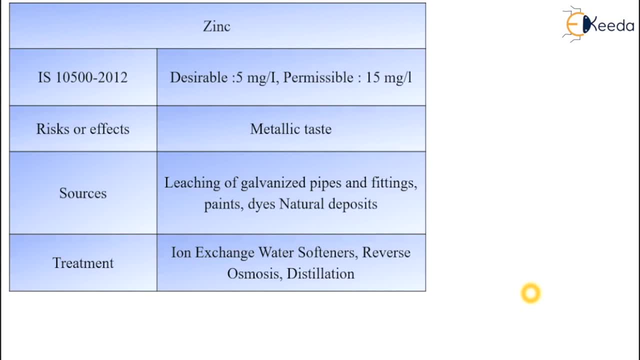 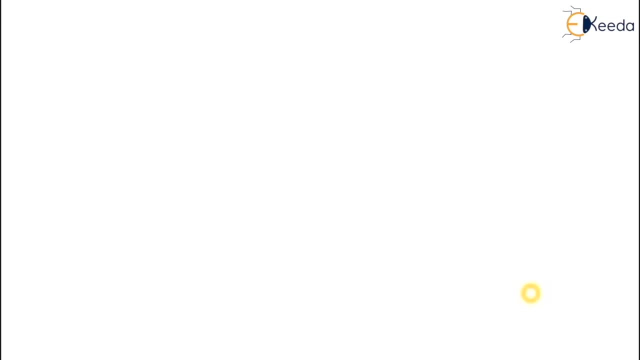 And treatment provided to remove the zinc as a heavy metal are The ion exchange method, water softeners, Reverse osmosis and distillation. So most of the heavy metals are removed by the process of ion exchange, reverse osmosis and distillation. 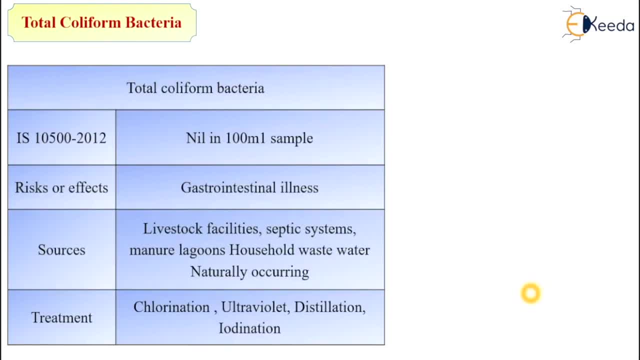 Then, in form of biological characteristics, we have to detect or count the total polyphorm bacteria, As drinking water doesn't contain these pathogenic bacteria, because it will be very harmful for the human body or spreading of diseases. So we have to detect this bacterial count and it must be zero in drinking water. 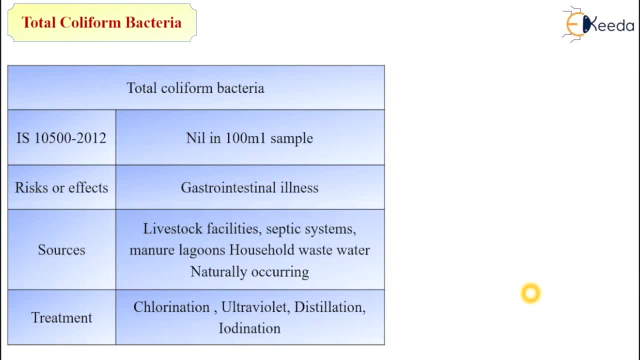 So, as per Indian standards, the total polyphorm bacteria should be nil in 100 ml sample And the risk or effects are gastrointestinal illness. Sources are livestock facilities, septic system, manure, lagoons, household water naturally occurring. 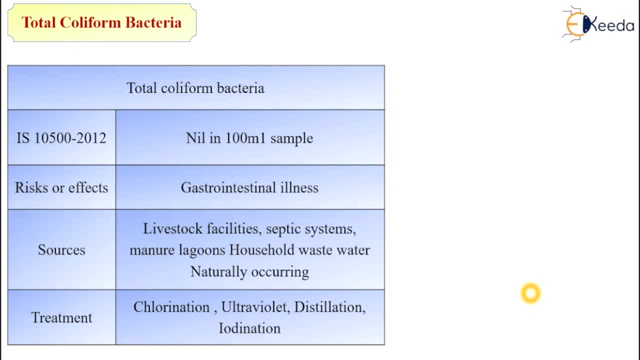 And treatments are provided in form of disinfection, Which includes chlorination, ultraviolet UV rays protection, distillation and iodization. Next is E coli bacteria. So, again, there are different types of pathogenic bacteria. One is in the form of total polyphorm bacteria and second one is E coli bacteria. 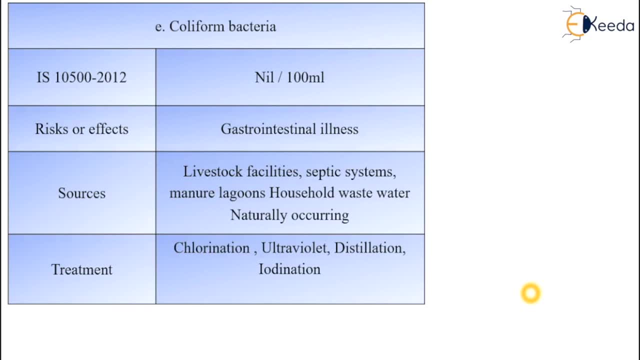 So again, as per Indian standard, the count of E coli bacteria present in drinking water source are nil per 100 ml of water. sample And effects are similar to the total count of bacteria. This is the total count of bacteria which is gastrointestinal illness. 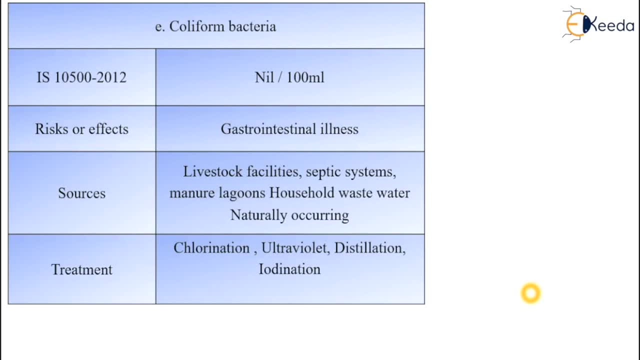 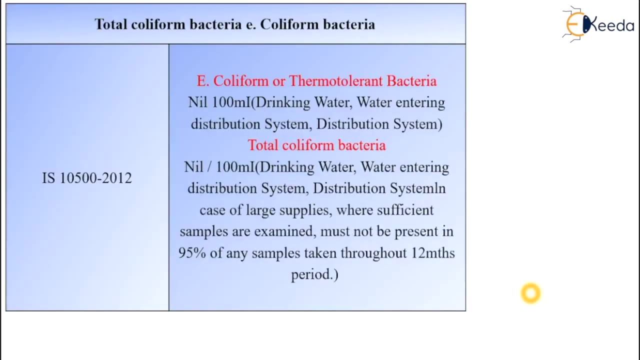 Sources also similar, That is, livestock facilities, septic system, manure, lagoon, household waste water naturally occurring And treatment provided in form of disinfection, Which includes chlorination, ultra violet protections, distillation and iodization. Next is Total polyphorm bacteria. 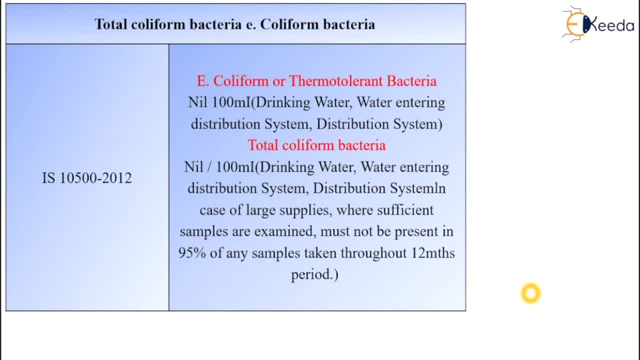 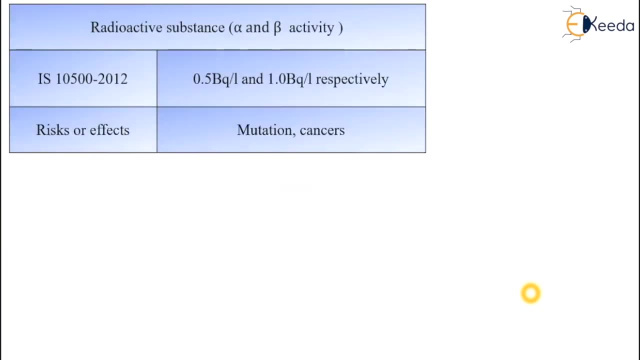 As per Indian standards standard, the E coli bacteria is nil per 100 ml of drinking water standards and total coliform bacteria is also nil per 100 ml of drinking water standards, as we have seen already in previous slides. and next is radioactive substances. so we are called it as alpha and beta rays.